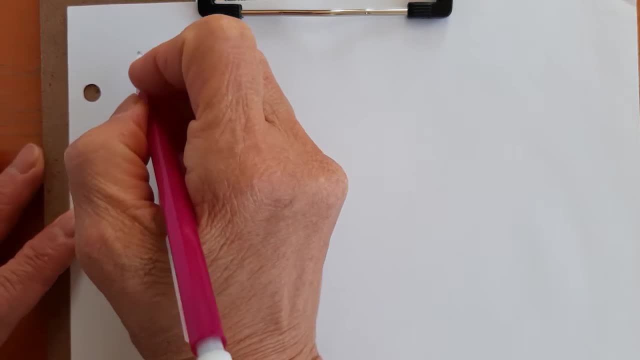 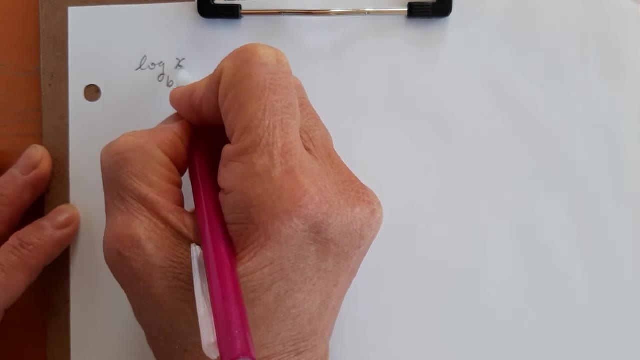 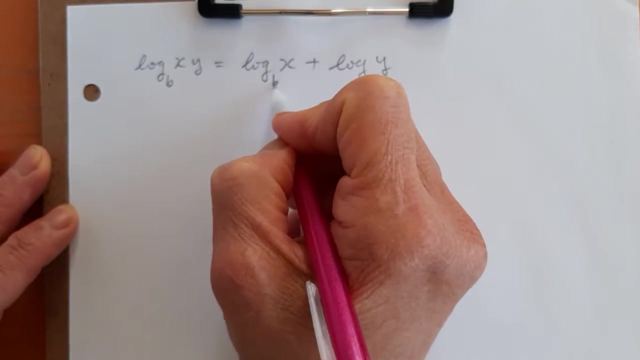 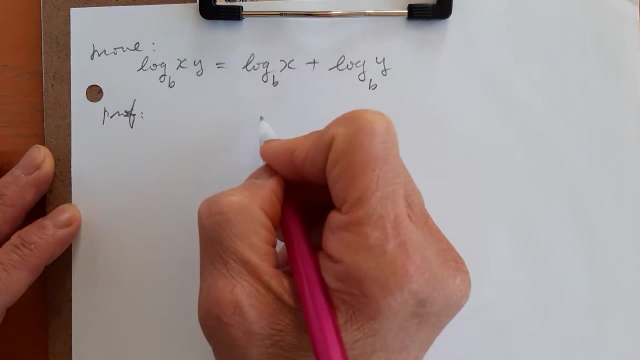 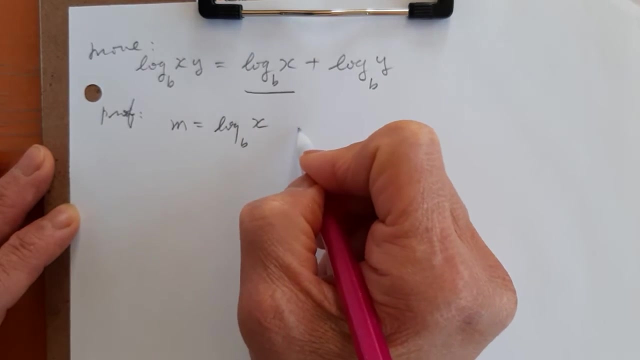 Prove the product rule of logarithmic function. Product rule is: log base is b x. y equals log x plus log y. Base is b. How to prove it? First of all, we let m equals log x and n equals log y. 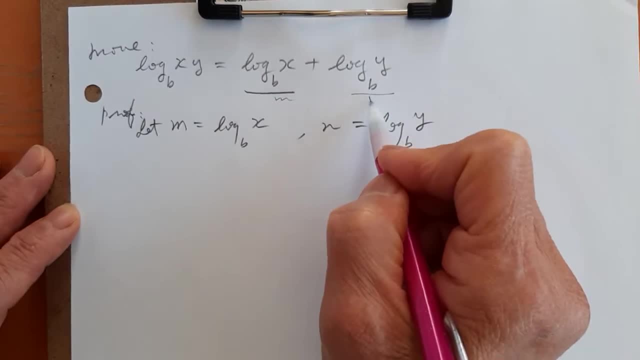 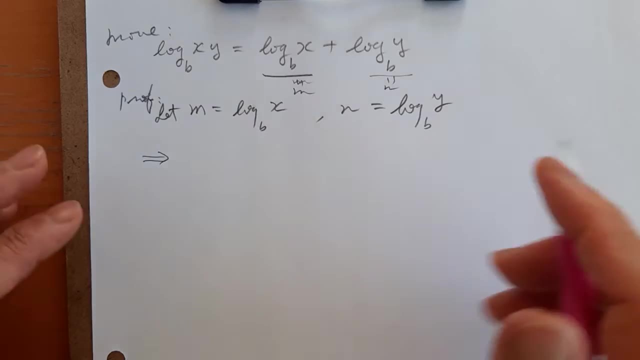 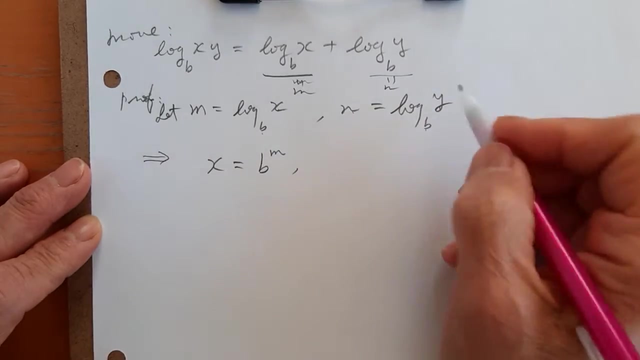 This is m, This is n. This equals n, This equals m. Then we can change to x Exponential form. b to the power m equals x, So x equals b to the power m. b to the power n equals y, So y equals b to the power n. 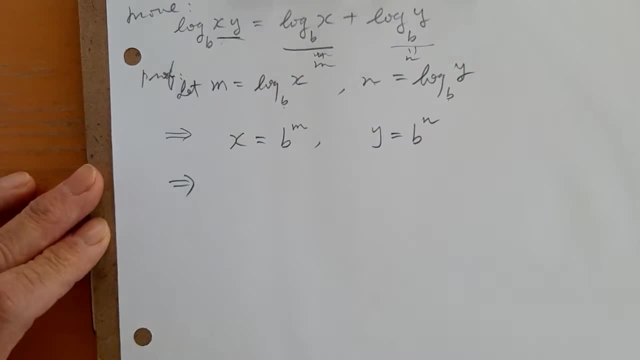 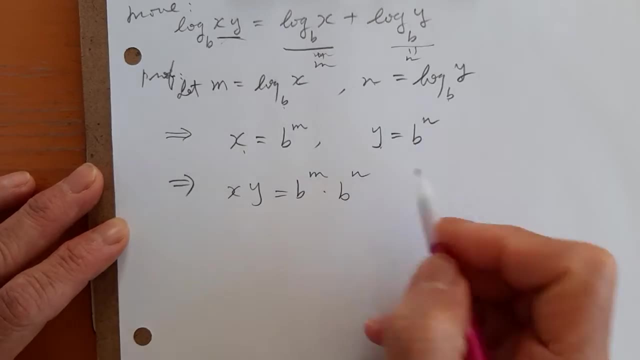 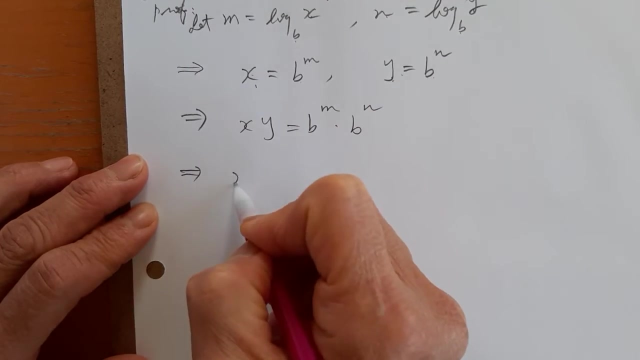 And then, since we are looking for x times y, so tying together, x is b to the power m, y is b to the power n- Left side tying together: x times y equals right side tying together, And then use the product. 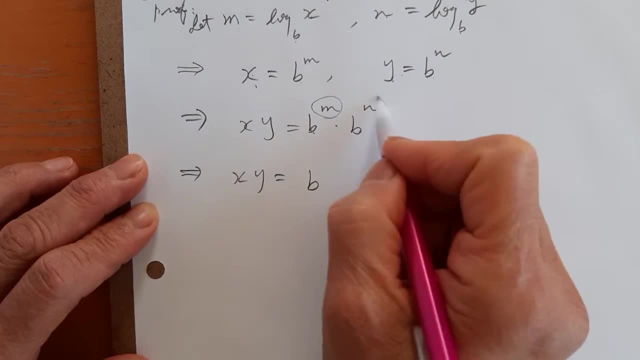 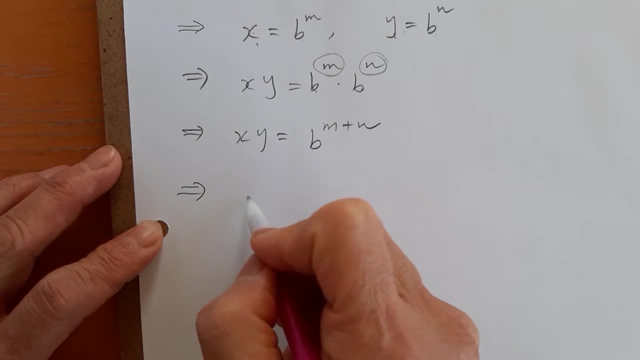 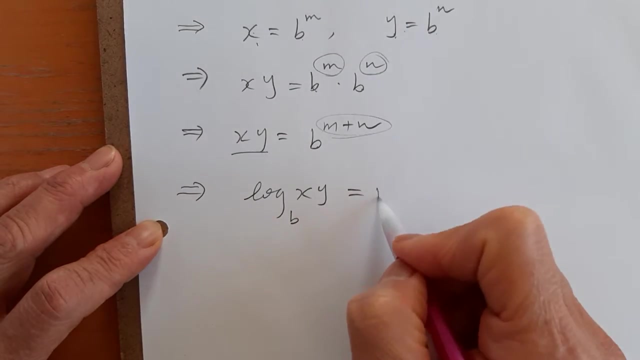 Prove the product rule of exponent. The same base is b. Add exponent m plus n, Then change from exponential form to logarithmic form. It's log base is b. function value x, y equals exponent m plus n, And so then plug back in. 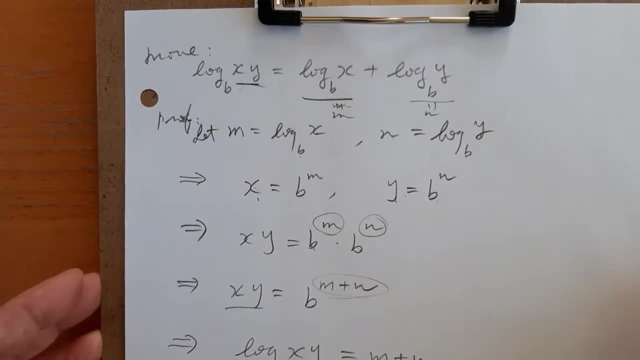 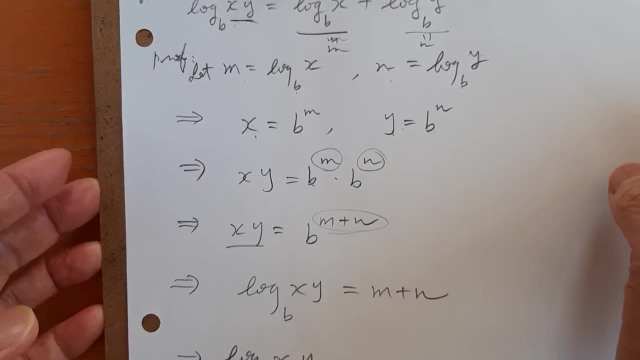 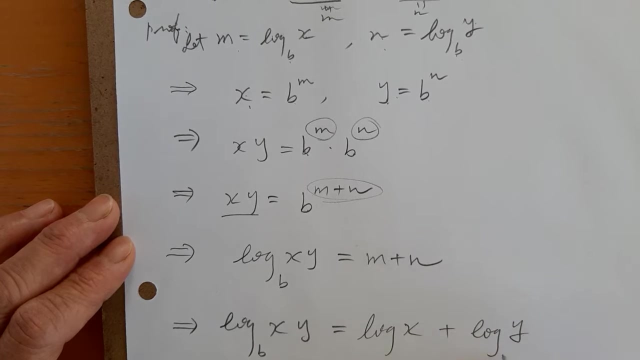 x y, log x y equal, Since we let m equal log x, n equal log y. So plug back in: m is log x, n is log y, base is b. Now we got proved, Get proved. 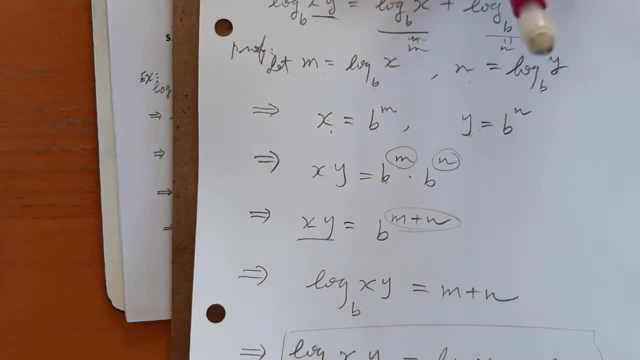 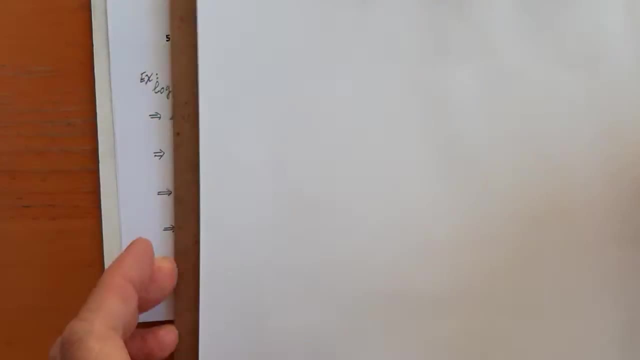 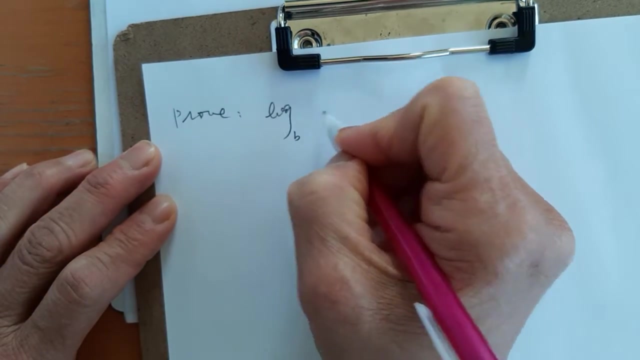 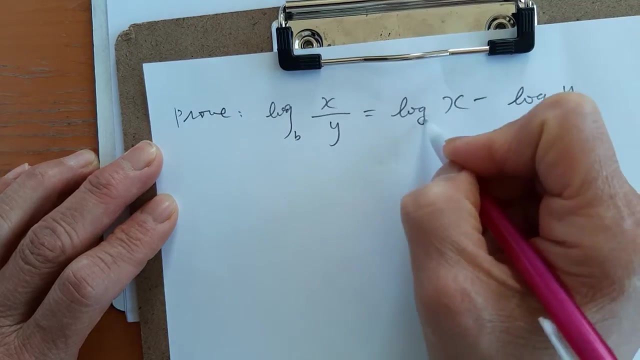 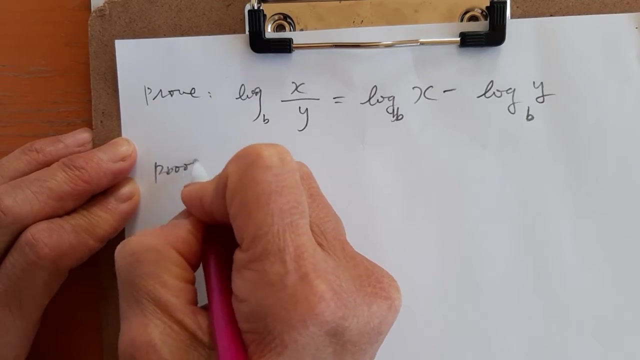 Product rule get proved. Then next is a quotient rule. Prove the quotient rule. It's log base is b. x over y is log x minus log y. subtraction base is b. Now how to prove it? And first of all, let this term, it's m. this term is n. 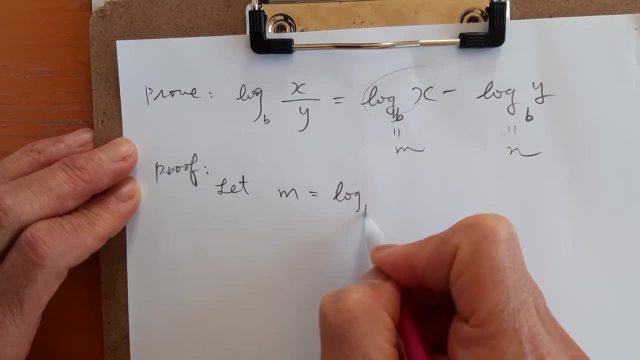 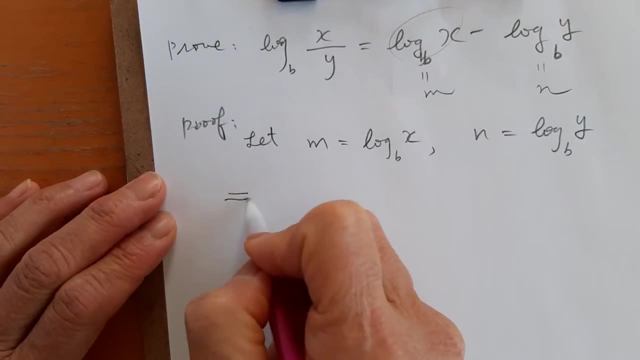 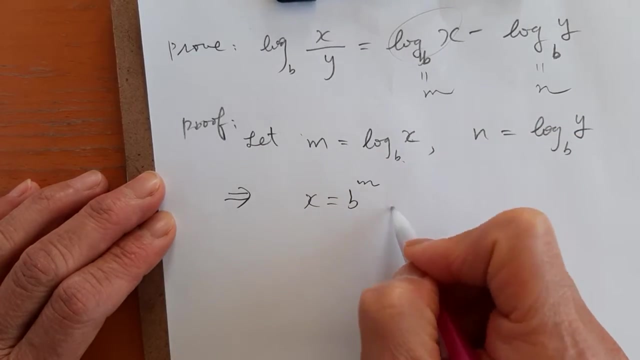 So let m equals log x, n equals log y And change from logarithmic form to exponential form. b to the power. m equals x, So x equals b to the power m. b to the power. n equals y, So y equals b to the power n. 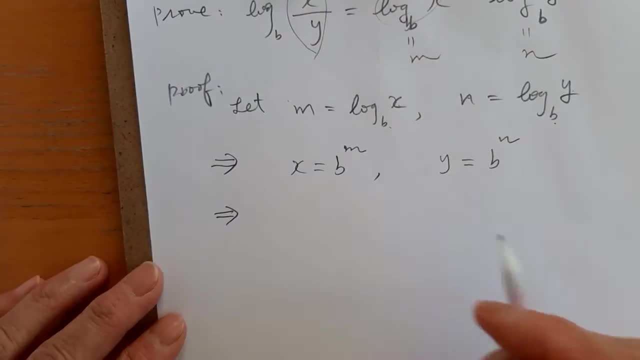 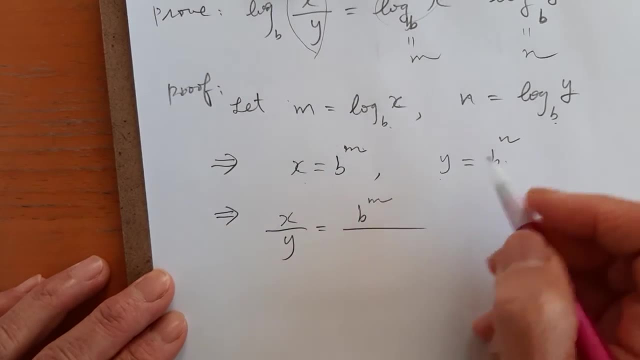 Then, since here we're looking for x over y, so divide x divided by y, x over y, And x is b to the power m, x is b to the power m And y is b to the power n. So left side divided by left side. 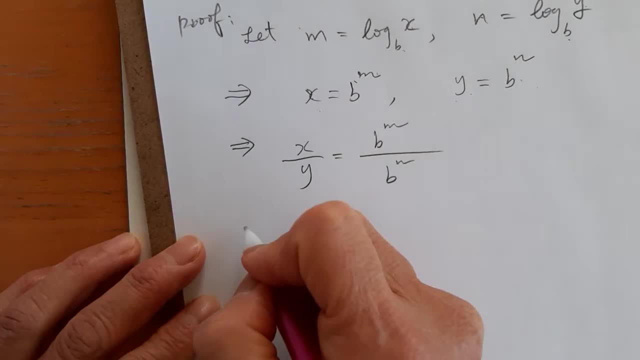 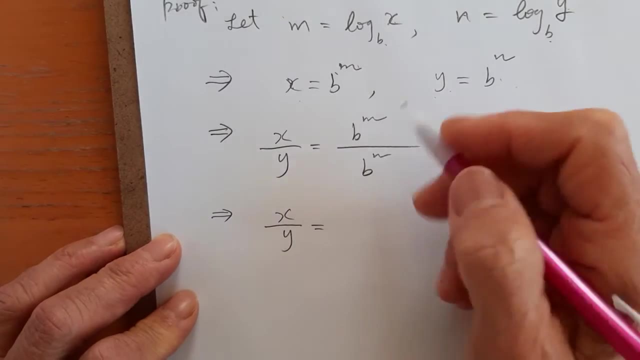 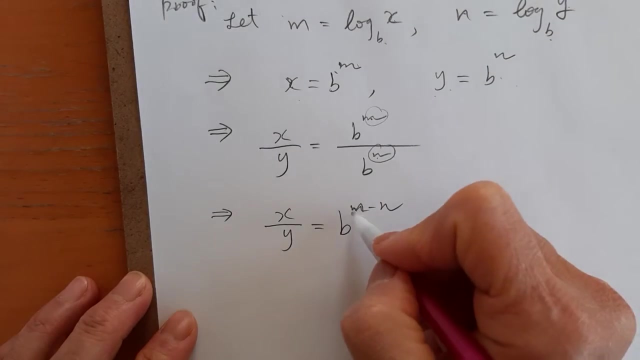 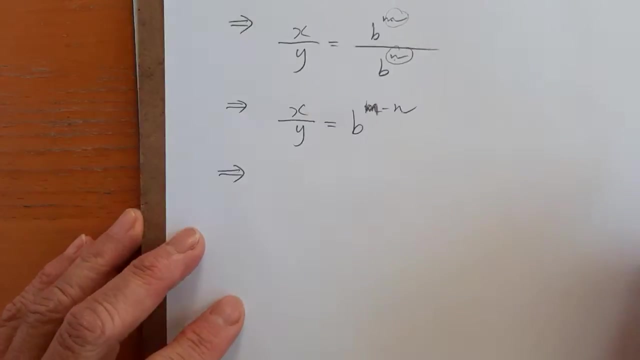 Right side divided. They are equal. And then use the quotient rule of exponent. The same base is: b You subtract exponent m minus n Subtract exponent. That's the quotient rule of exponent, Subtract exponent. And then change this exponential form to logarithmic form. 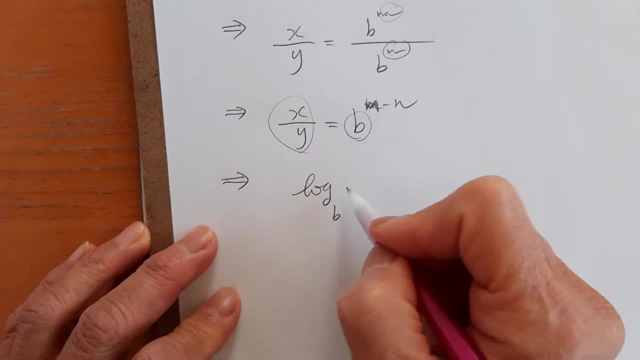 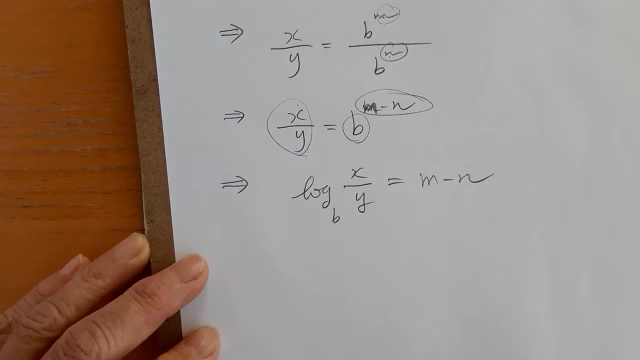 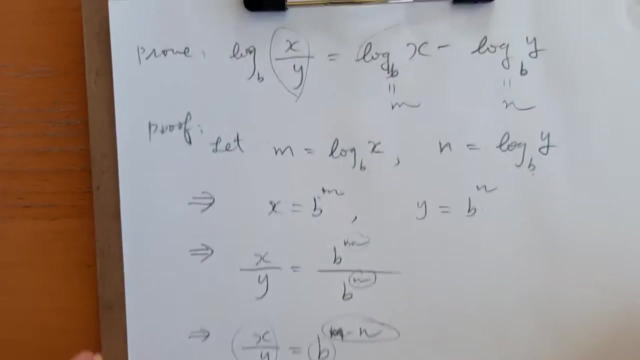 Base is b. Function value. Exponential function value is x over y, Equal exponent m minus n. Then base b: x over y. What is m? Because we let m equal log x, n equal log y. So plug back in. 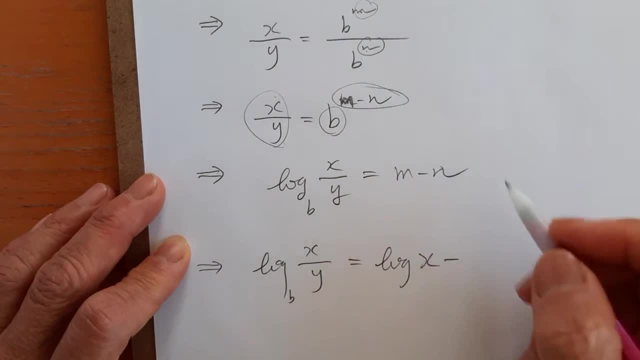 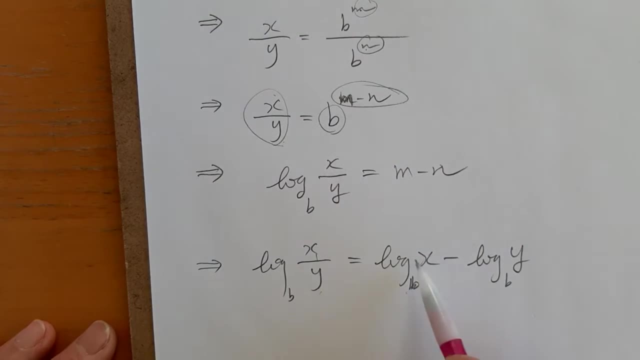 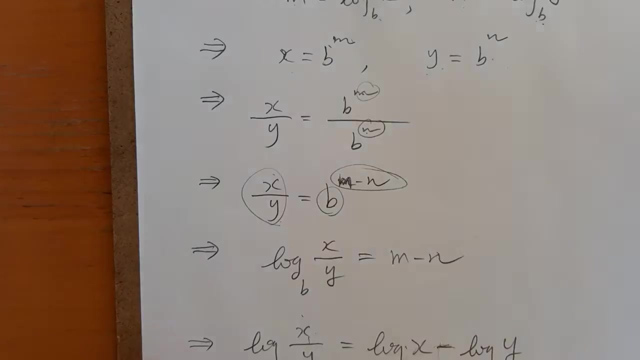 m is log x, n is log y, n is log y And base is b. And we got proved: Quotient rule is subtraction, Product rule is addition. Quotient rule here is subtraction. So we got proved. So we got proved. 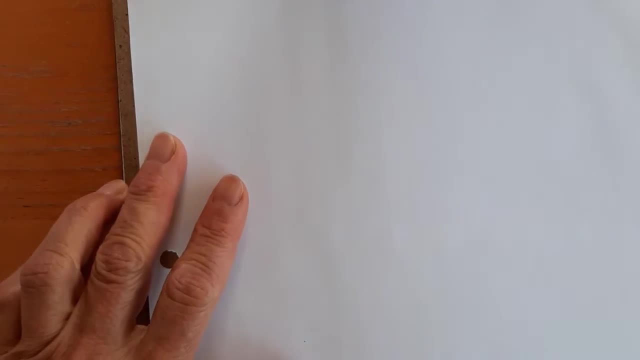 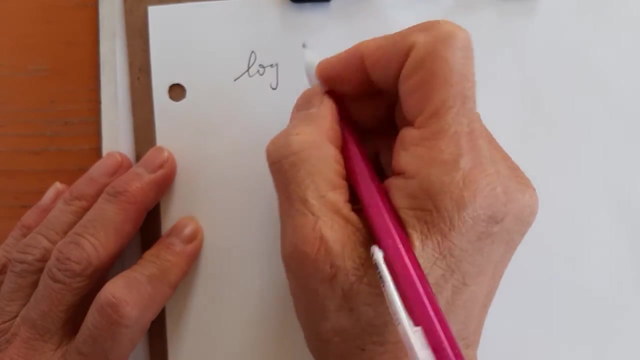 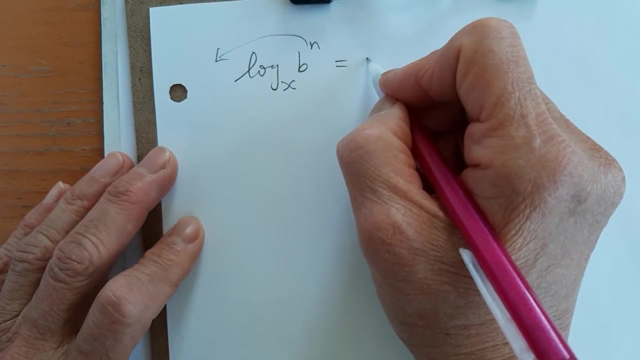 And then we can prove the power rule. The power rule is. The power rule is. The power rule is: log b to the power n equals b to the power n equals n. you can go from n. you can go from n. log base is. log base is. 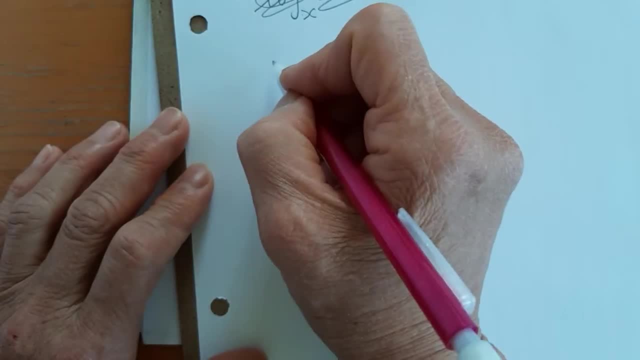 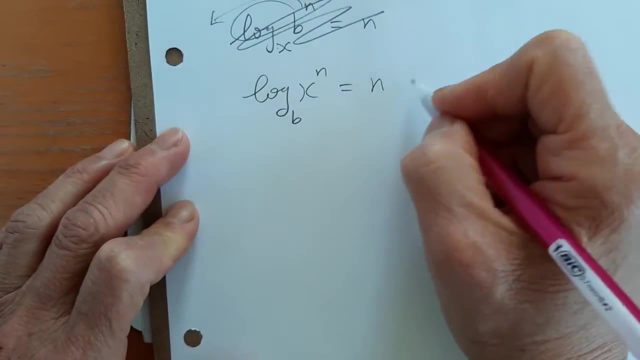 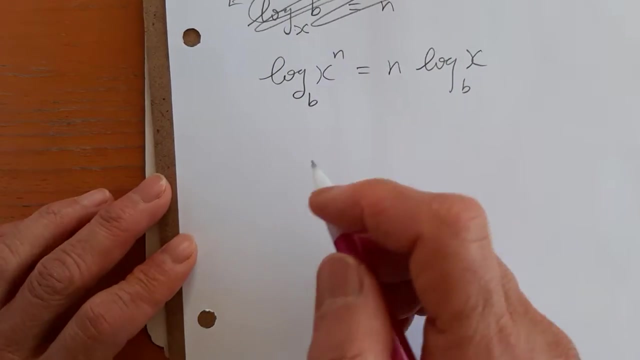 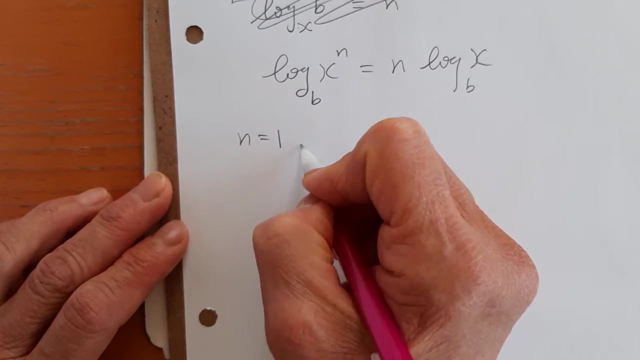 Let's put this way. Let's put this way: Log base is b x to the power. n equals x to the power. n equals n. log b b x. So How to prove this? How to prove this: If n equals 1, then 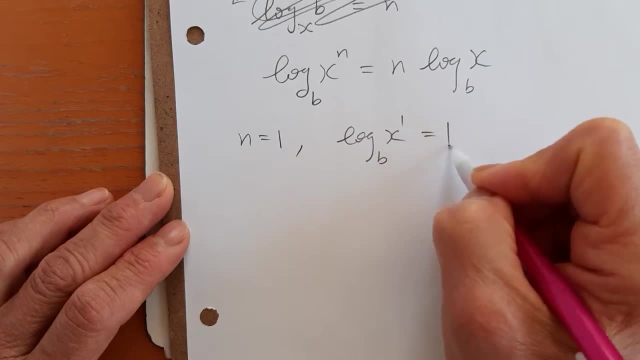 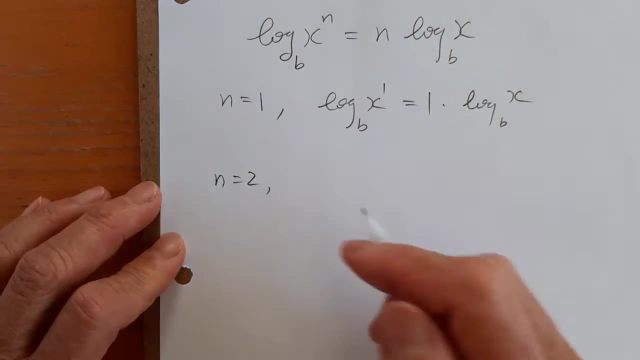 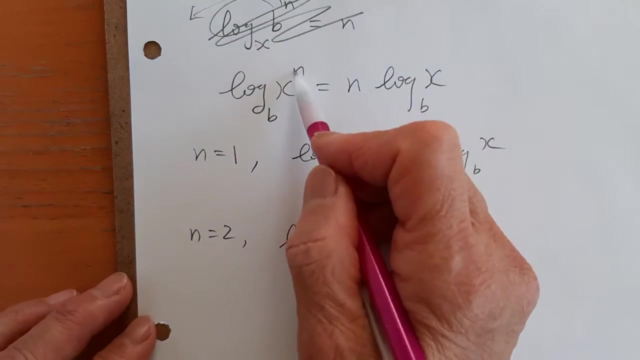 the left side is log base. log x to the power n equals right side Equal. They are equal. No problem If n equal 2. If n equal 2, log base is b x squared log base is b x squared 2 to the power n. 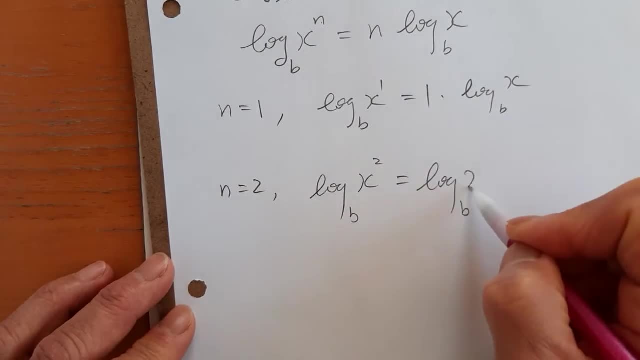 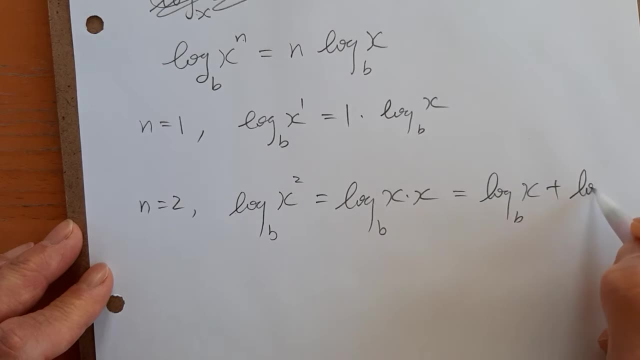 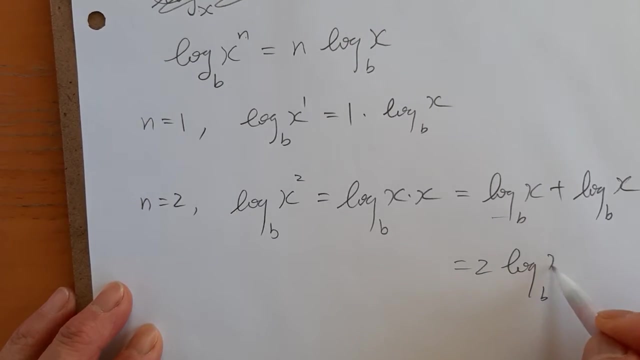 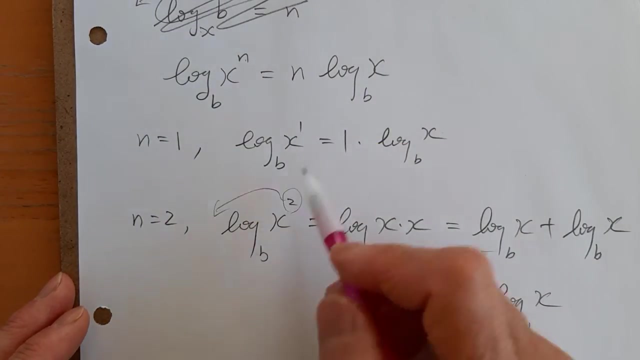 That is equal, that is equal to log x times x. and use product rule, you can get log x, You can get log x, log x and the two are same. add together is twice log x. So when n equal 2, n equal 2. So When n equal 2. 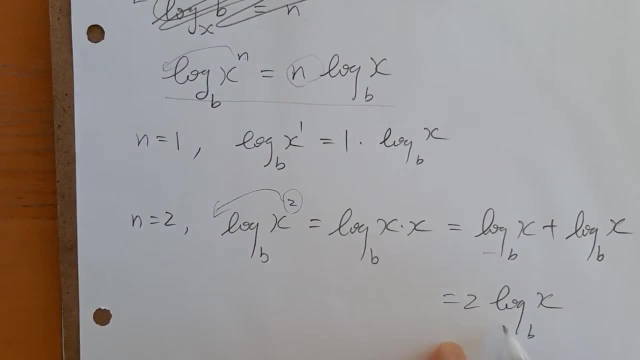 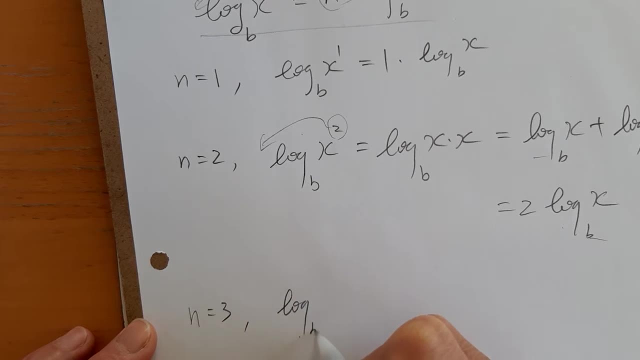 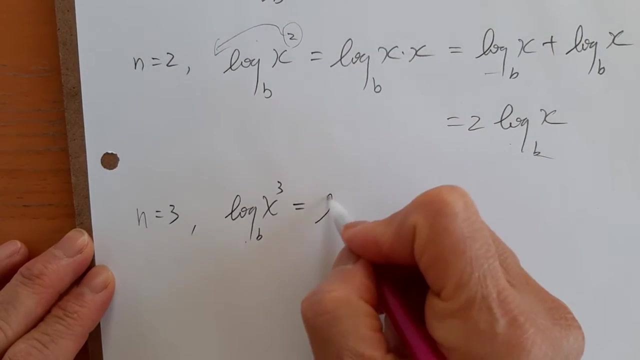 front. you got this general rule. so n equal 2 is a is a true is true. then you can prove. find n equals 3. when n equals 3 is a log x cubed and there's a 3, plug it in and that it will be equals log x squared times X, basis B and use product. 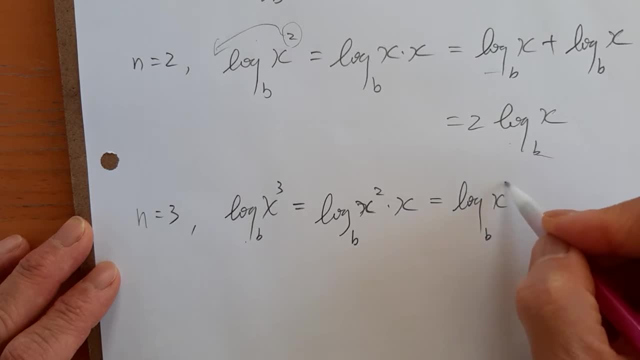 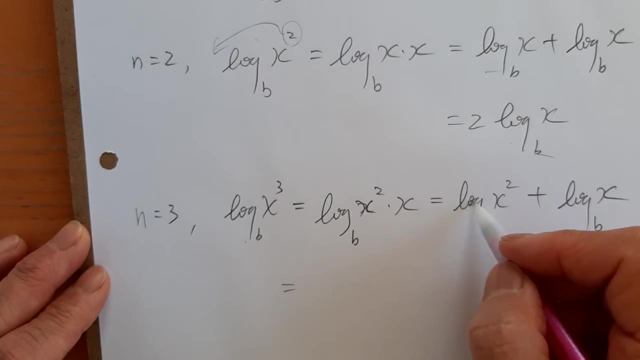 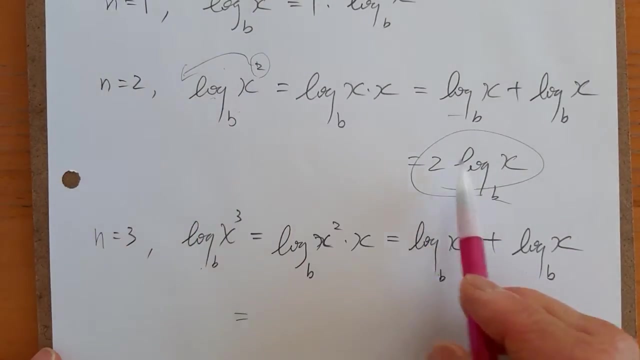 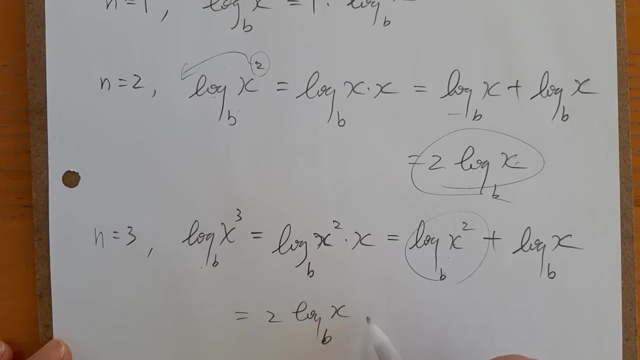 rule again, that is, a log x squared, add log X. and since log x squared, we already got from previous one, when n equal 2, we got log x squared equal to log X. so this log x squared equal to log X, and you add this one more, one more log X. 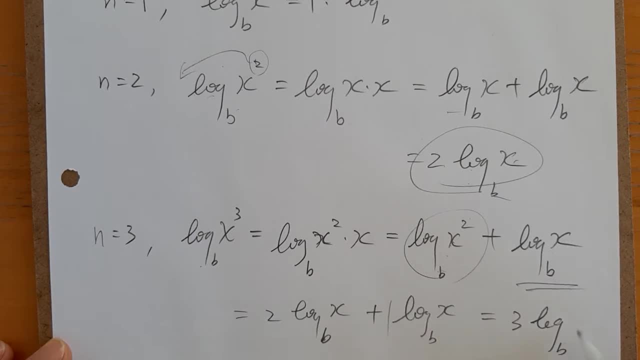 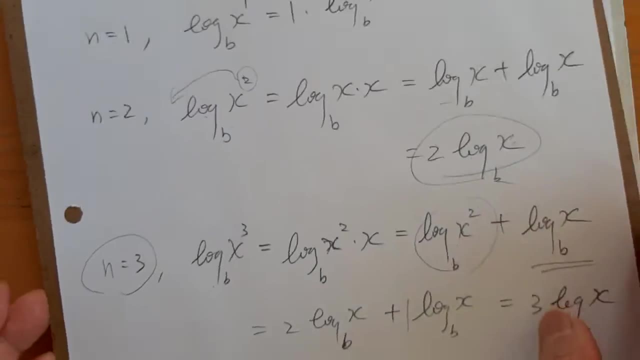 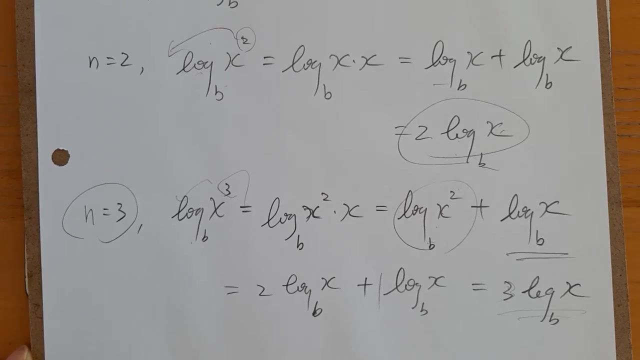 and totally 3, I log x. so when n equals 3, this also true when n equals 3, here is 3. when n equals 3 and then 3, move to the from and you got 3, so and etc. you can prove. so that means when: uh, and that means 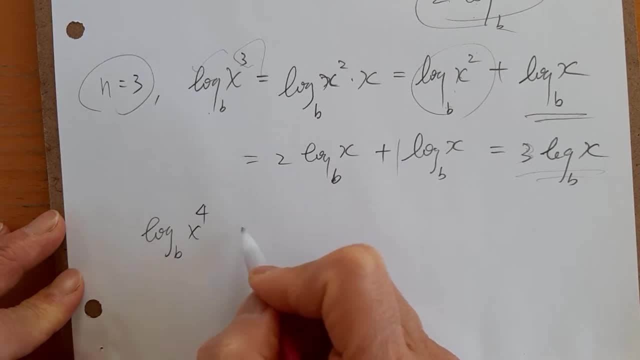 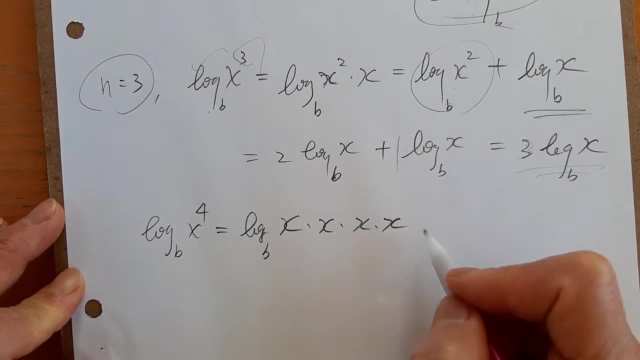 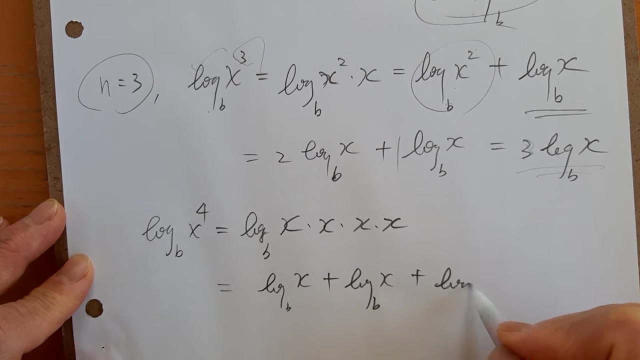 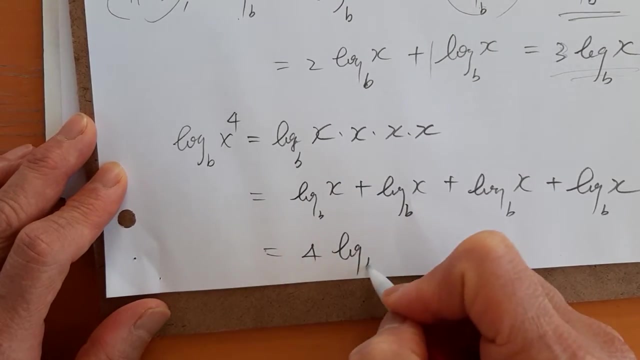 when log b x to the power 4, that is a log b x times x times x times x and you can write as a log x plus log x plus log x plus log x and that is equal 4 log x. so if n, then you have n log x. 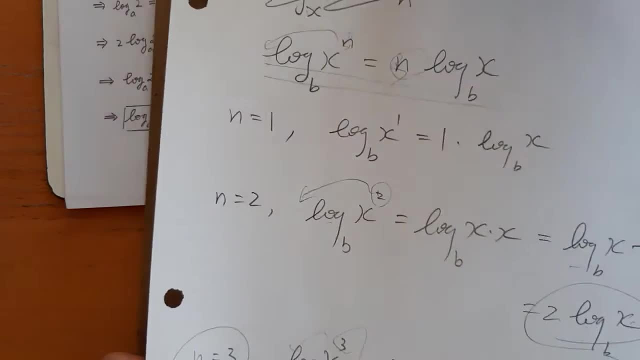 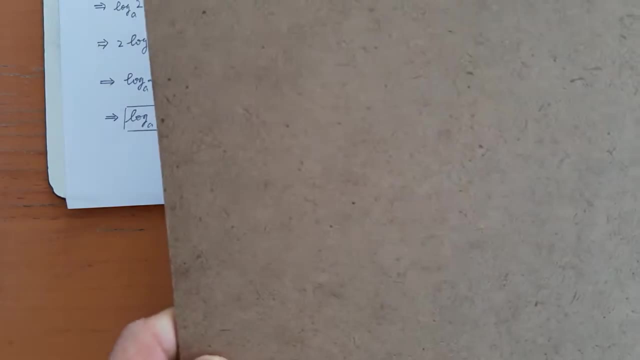 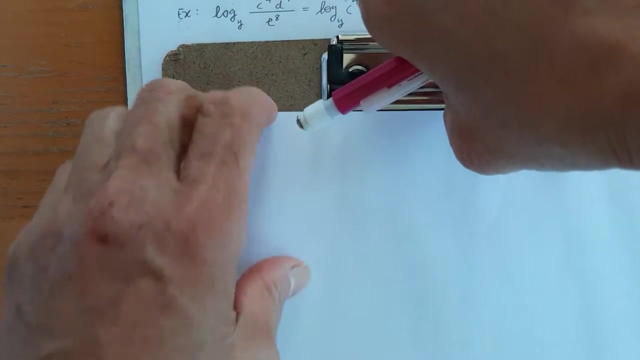 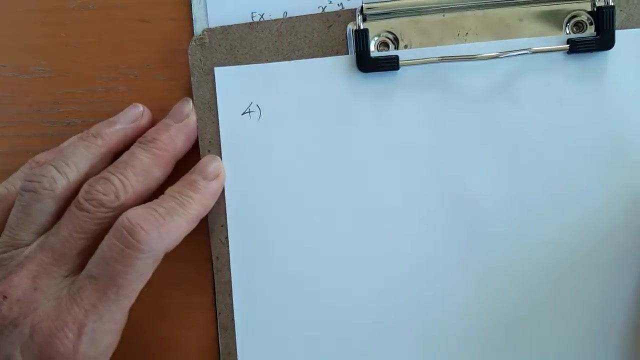 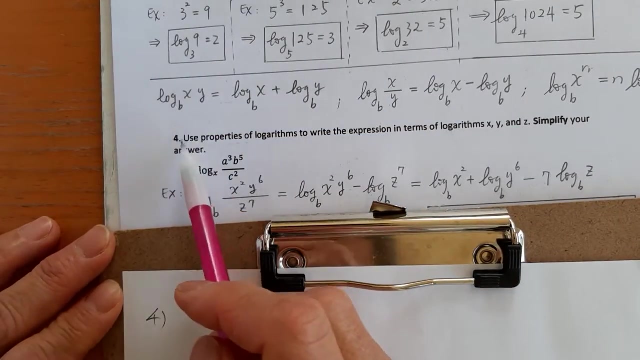 all right, this is a power rule. a power rule, uh, then. uh, now let's try some uh questions. that's your uh homework example. homework question four example: uh, four, um, this use the um here's started using a bit of technology. um, heres the two team thing we 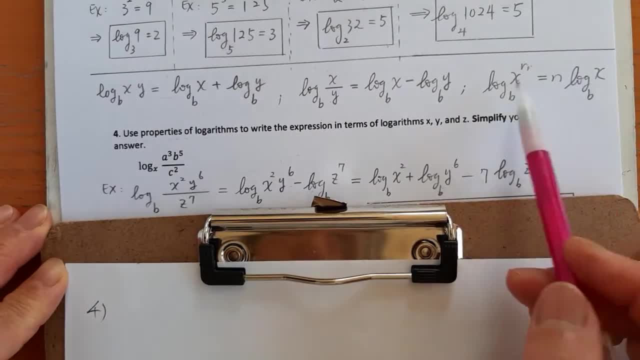 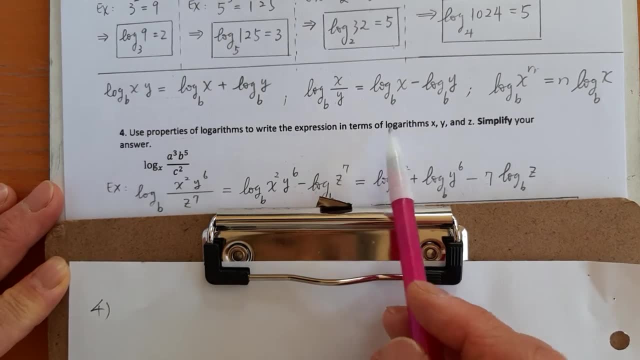 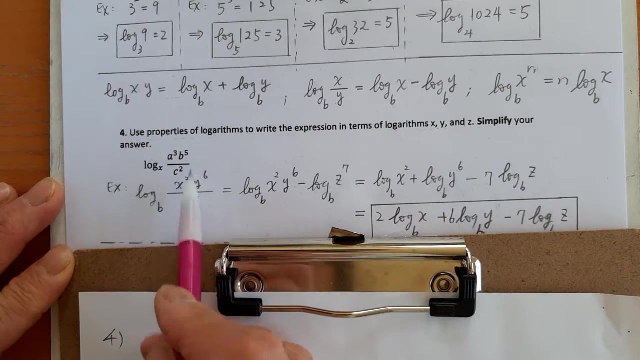 just talked about here, um, before this, how i write down product rule, quotient rule, uherv, uh, power, power rule, power rule. and question four: use properties of logarithm to write the expression in terms of logarithms x, y and z. simplify your answer and this is your home work question. let's try this example: career. 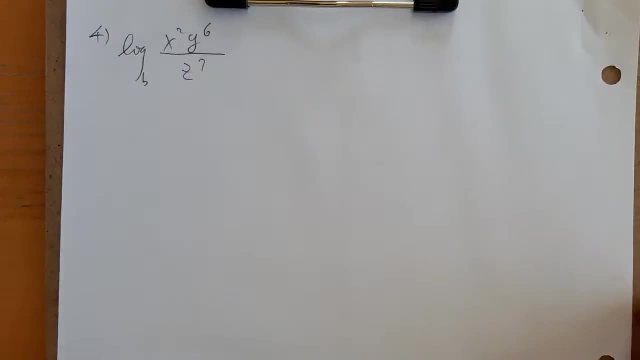 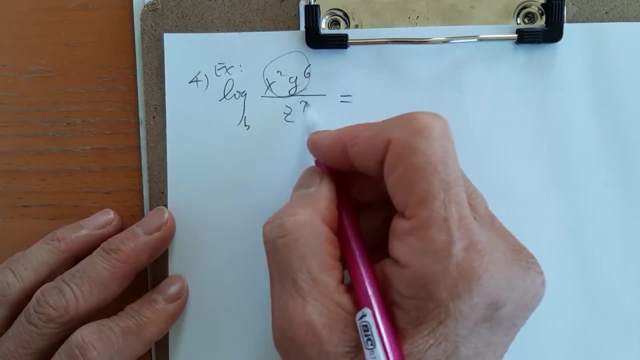 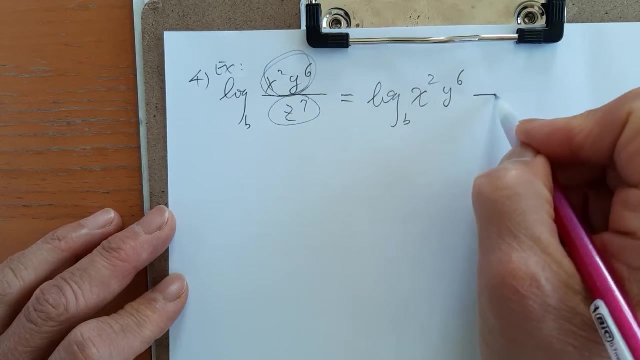 y to the power of 6, z to the power of 7.. This example is an example for your homework, question 4.. So, first of all, use quotient rule. This is divided, So use quotient rule. is log numerator, subtract, log denominator. 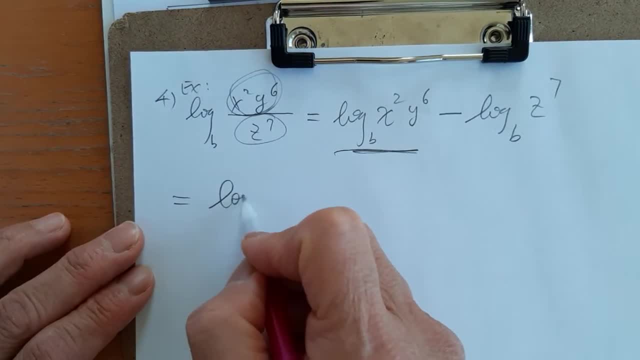 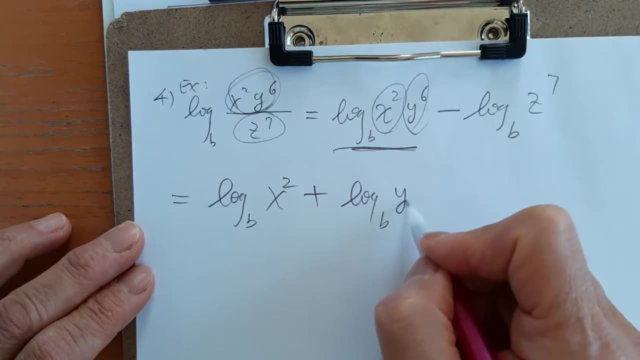 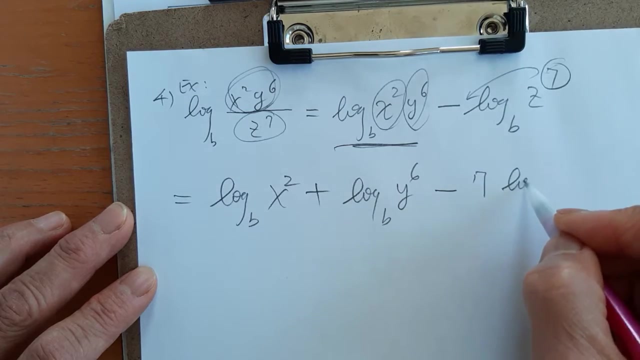 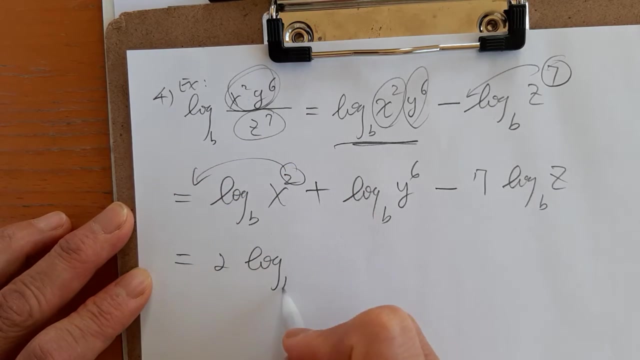 And then this is product rule. You got log this. add log second one. then and this: use power rule This: 7 go from 7 log z And continue. use power rule This: 2 go from 2 log x plus 6. go from 6 log y minus 7 log. 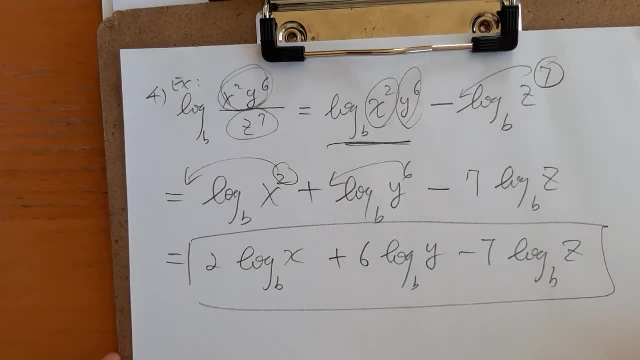 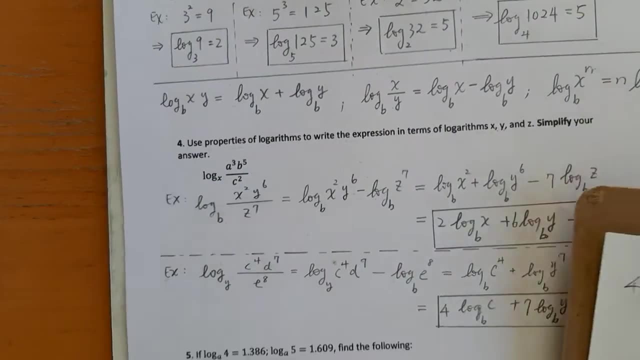 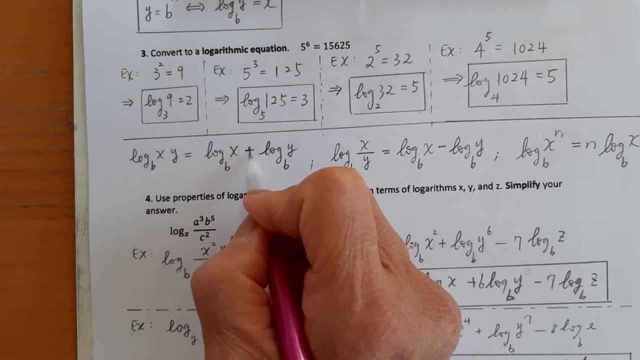 So, after use, go right in terms of log of x, y, z, That's, use the properties, use those rules If a product here is addition, If a quotient here is a subtraction, If a 2d power n n go from. 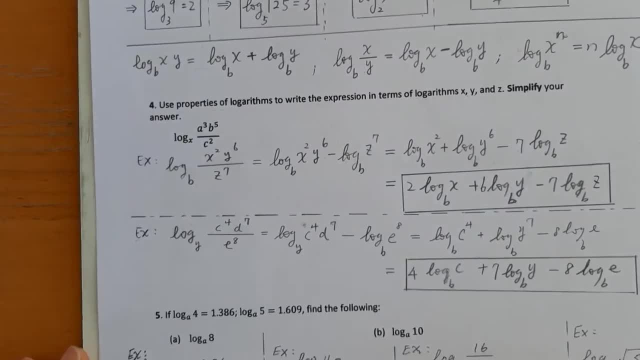 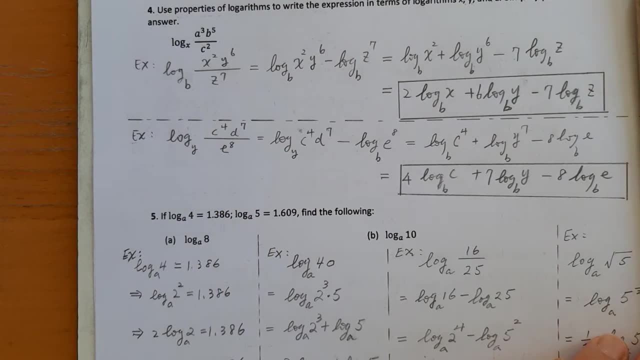 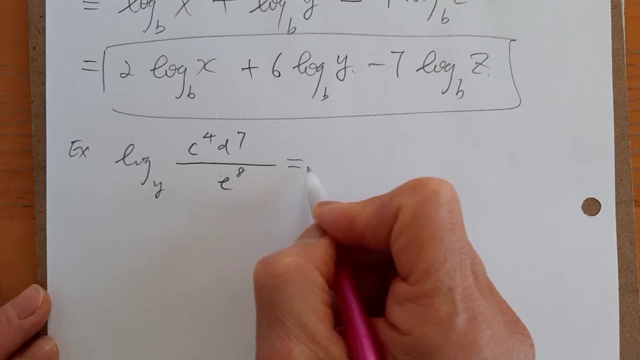 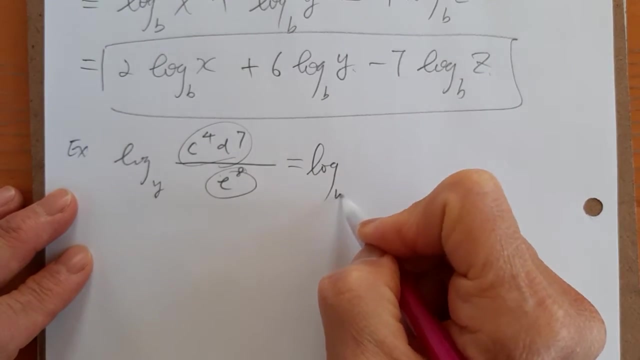 Product rule, quotient rule, power rule. Let's try another examples. this example, Example log y, c4,, d7,, e8,. this example, this, So do the- is numerator divided by denominator, So use quotient rule. log y is the base numerator, c to the power of 4,, d to the power of 7.. 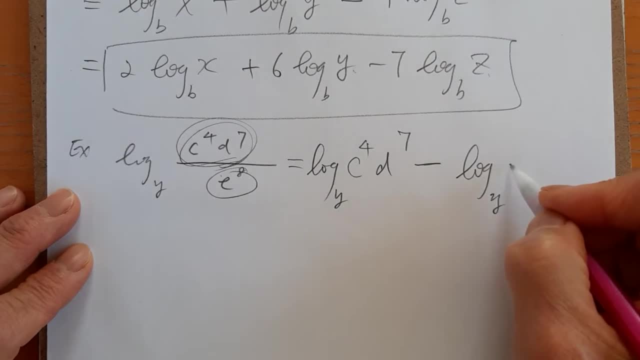 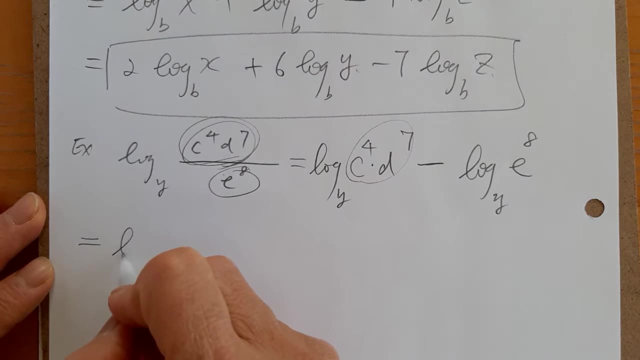 Do subtraction log y, e to the power of 8. Then this is a multiplication. so use product rule And get log c to the power of 4, add log d to the power of 7.. The base is y. 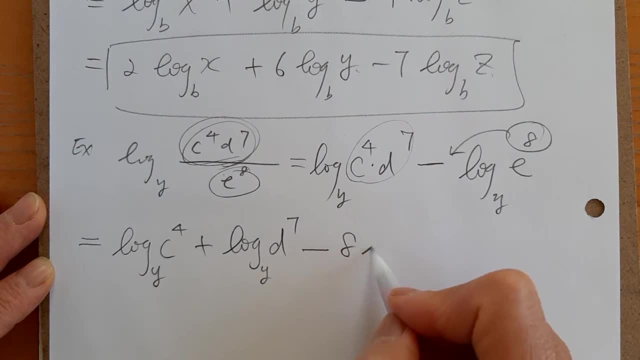 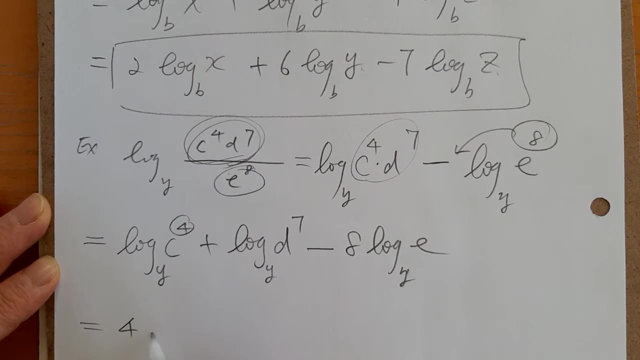 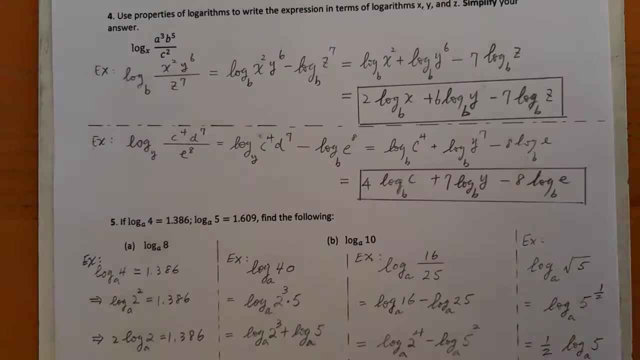 Minus this use power rule 8 go from 8 log e, And then this use power rule 4 go from 4. Log c plus 7 go from 7. log d minus 8 log e. That's we write as simplify it. 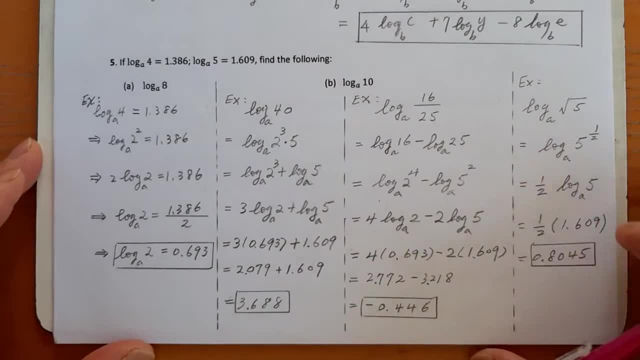 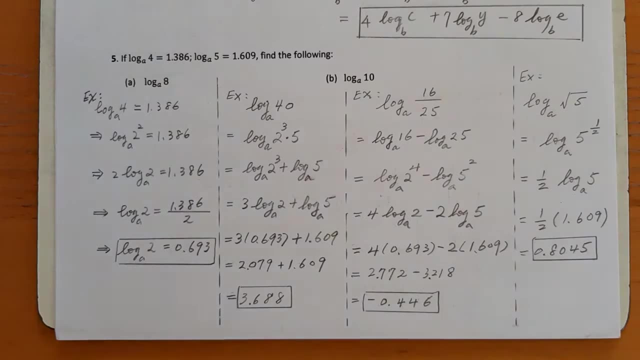 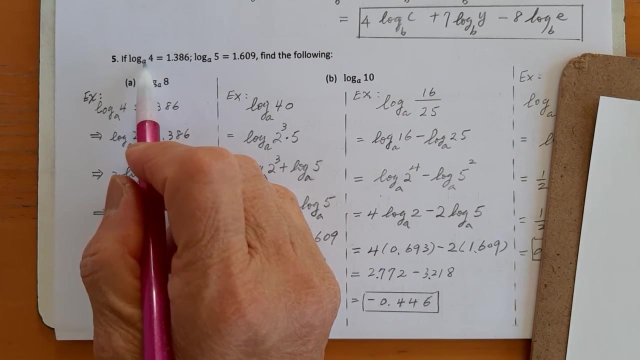 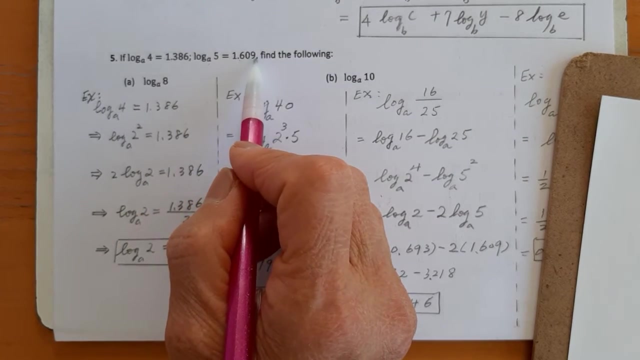 Now question 5.. We also use product rule, quotient rule and the power rule to do To do Question 5.. Question 5. Given log base is a4, equal 1.386.. Log base is a5, is equal 1.609.. 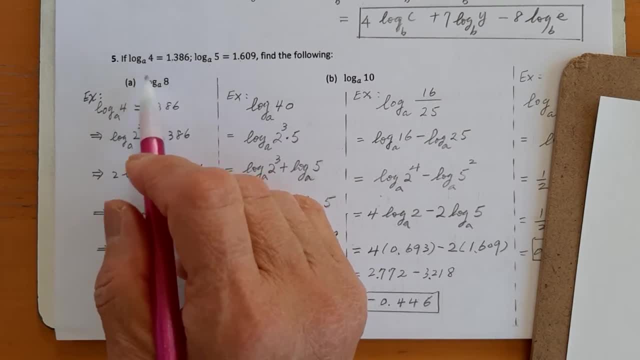 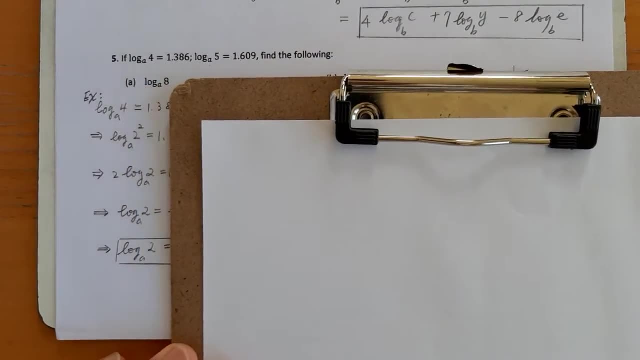 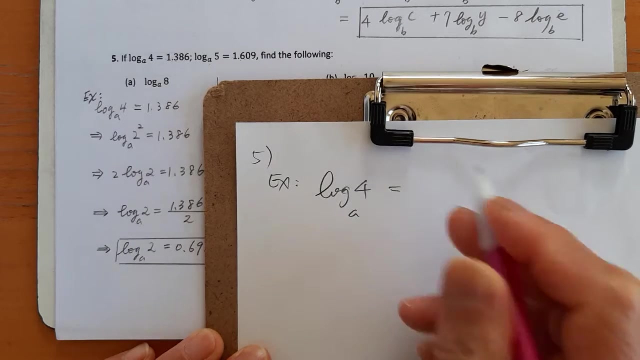 And figure out: a- this is your homework question- and log 8, and log 10,: a and b, That's your homework question. Now let's try example. This is question 5.. Example: looking for log This one, log 4.. 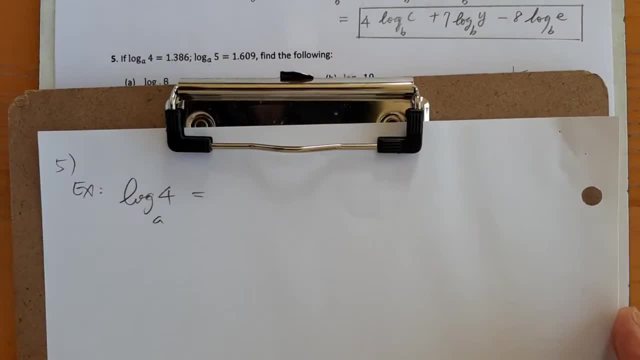 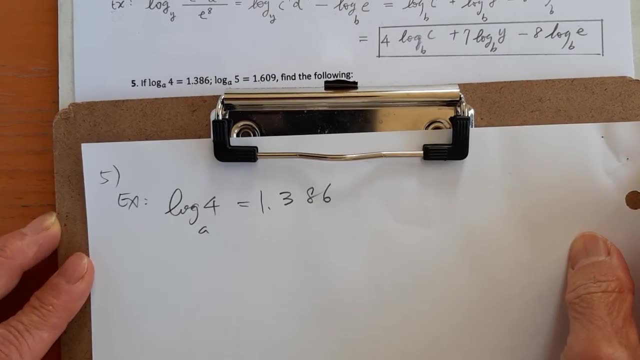 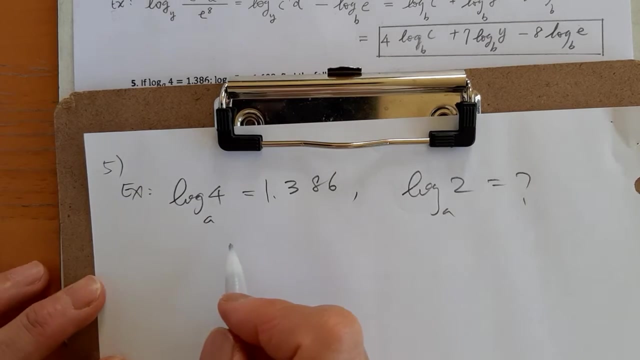 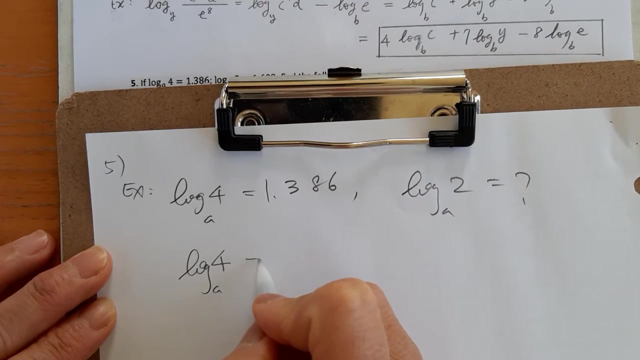 Looking for log 2.. So, since given log 4 is given is 1.386.. It's already given, question already given. Now ask you: what is log 2?? What is log 2? Since log 4 is 1.386.. 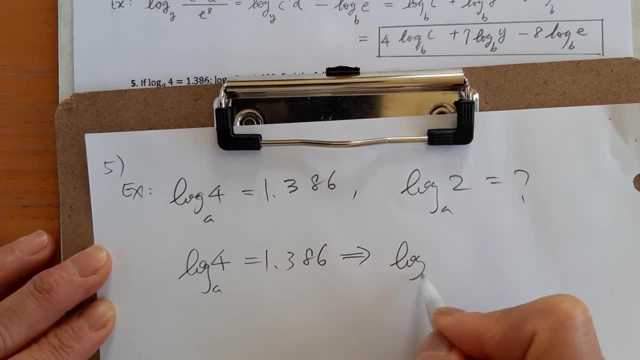 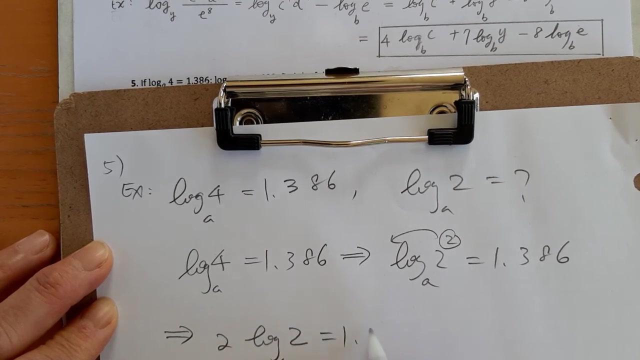 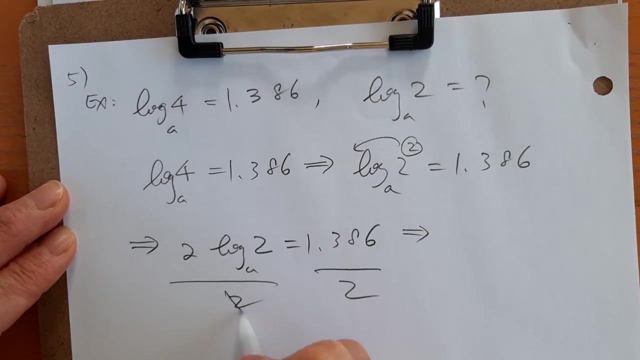 And log 4 is: 2 squared equal 1.386, and use power rule this: 2 go from. So you got 2. log 2 equals 1.386,, 2 go from. Then you divide it by 2, both sides 2 cancel. 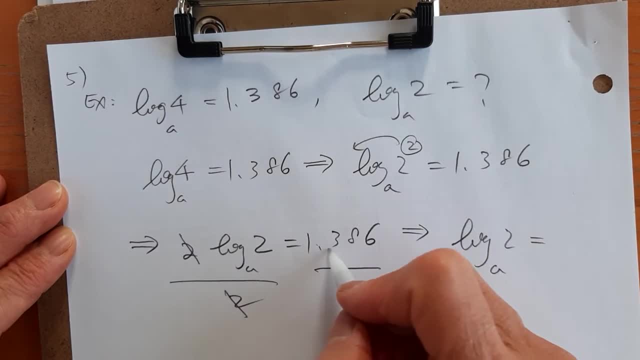 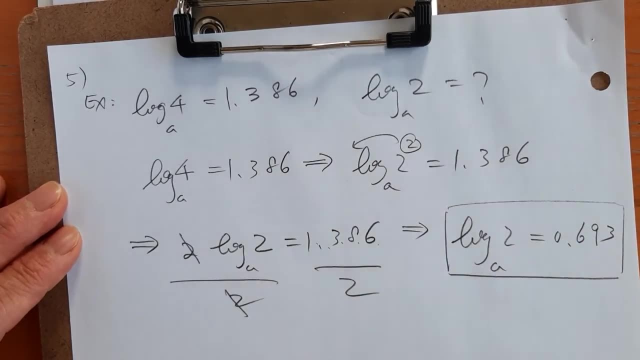 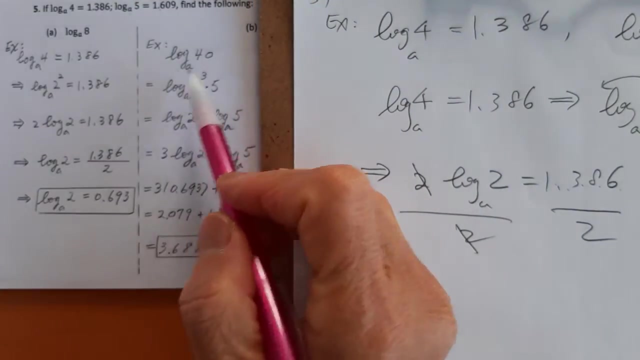 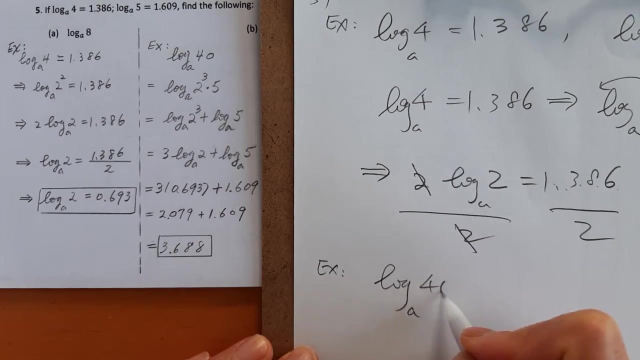 So you log 2 equals 1.386.. 1.386 divided by 2 is 0.693, and you got log 2.. Now and example. next example Log 40.. Example: log base is still a 40.. 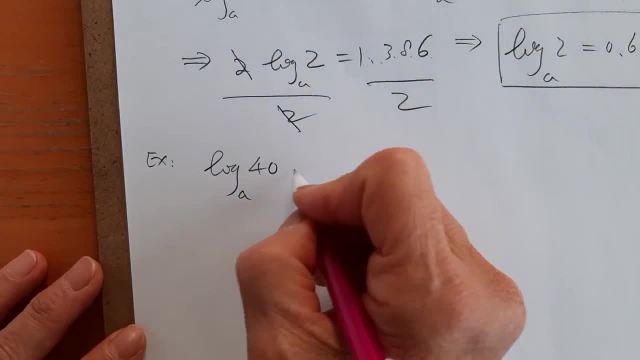 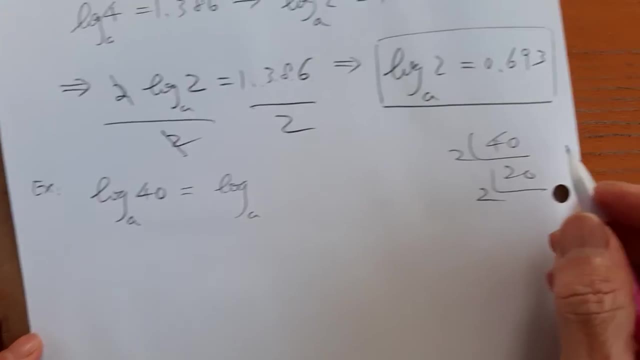 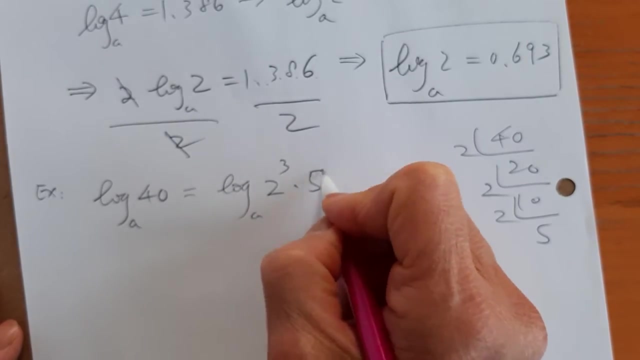 Now, since 40 is equal to 40, you can divide it by 2.. Get 20 divided by 2,. get 10 divided by 2, get 5.. So 40 is 2 cubed times 5.. 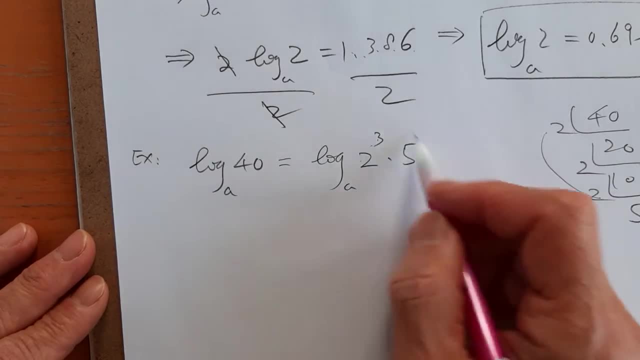 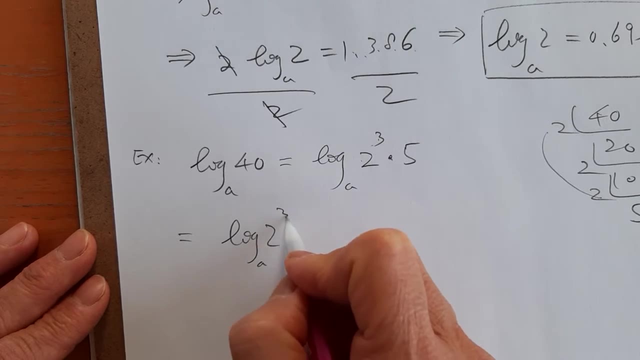 2 times 2 times 2 is 8,, 8 times 5 is 40. And since you can, this is product, So use product rule. You got log 2 cubed. add log 5.. Product rule. 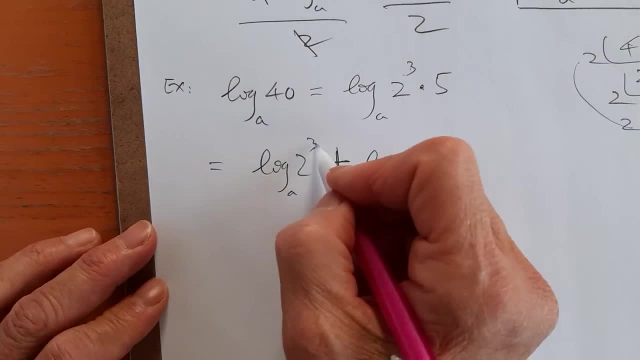 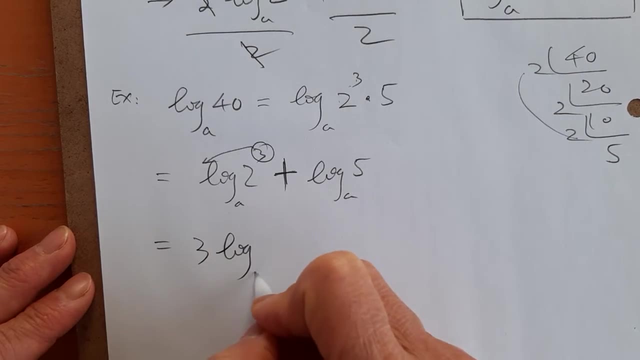 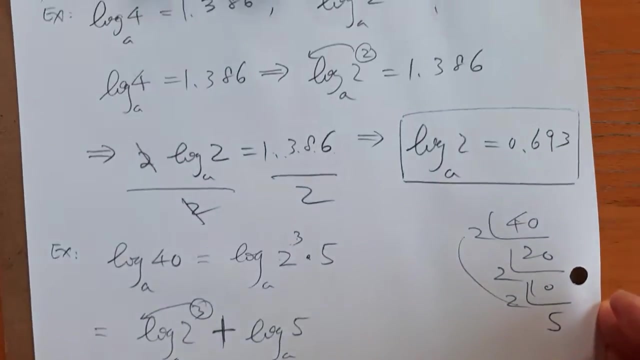 Here is the product. Then you add: Then use power rule, This 3 go from, Now 3 go from. So you got 3 log 2, add log 5, 3.. Now log 2, we already find in previous example- is 0.693.. 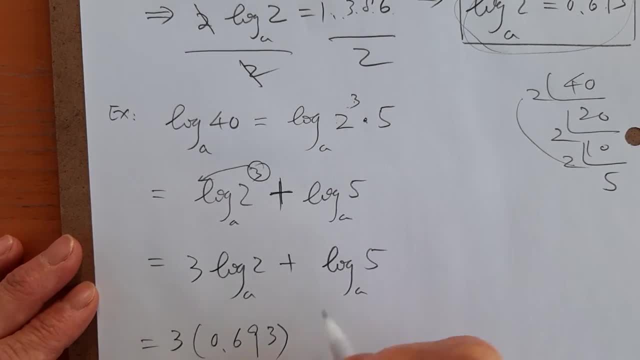 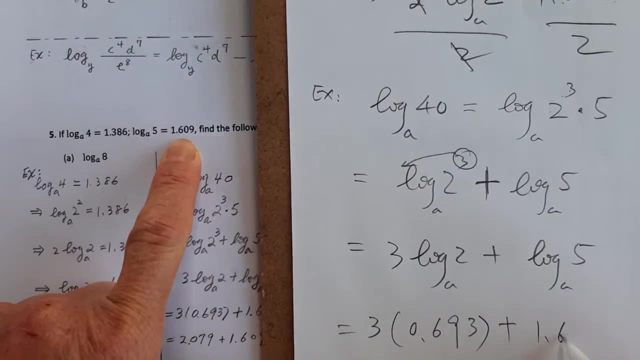 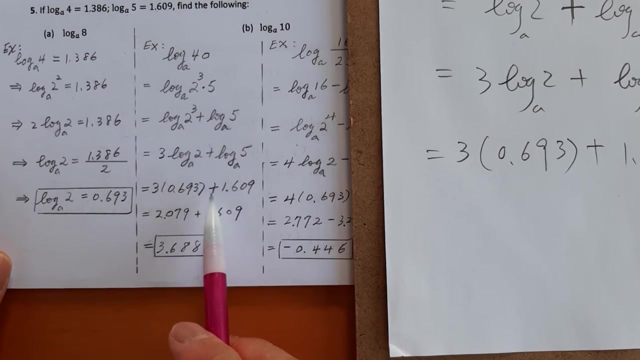 So it's 0.693.. Add log 5.. Question given log 5, here It's 1.609.. 1.609.. So you will get is 3.0693.. Add 1.609.. 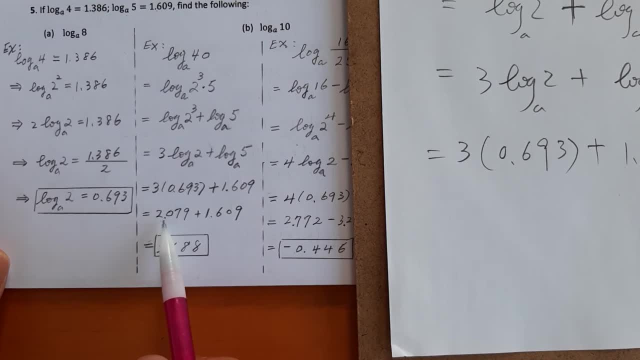 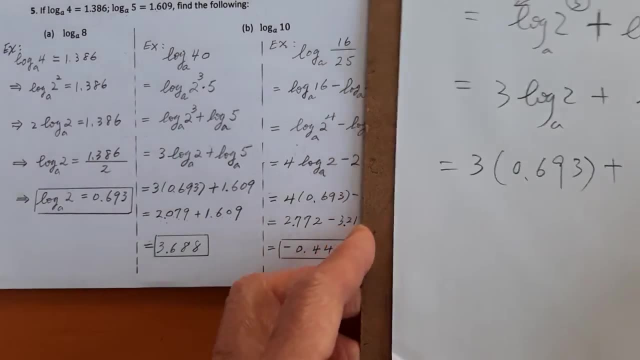 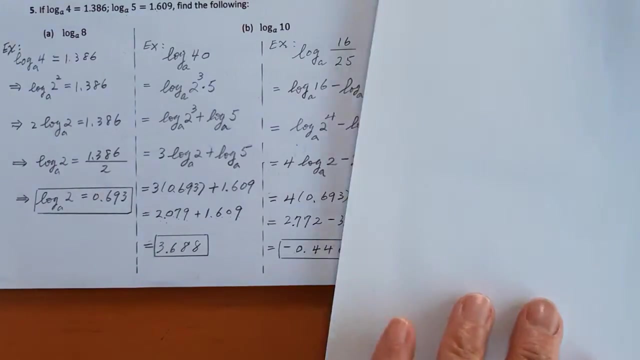 3 times. 3 times 0.693.. Got 2.079.. Add 1.609.. Add together is 3.688.. That's another example. Next example: it's use quotient rule. example: This one, this example. 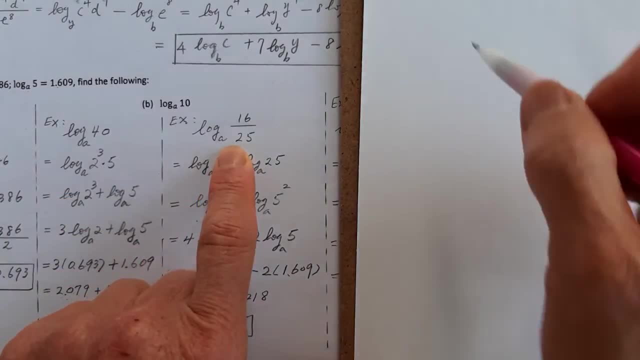 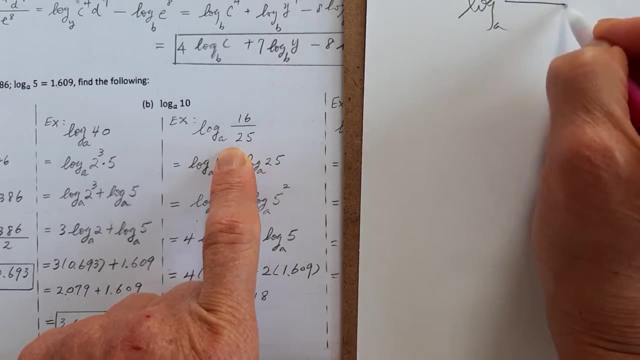 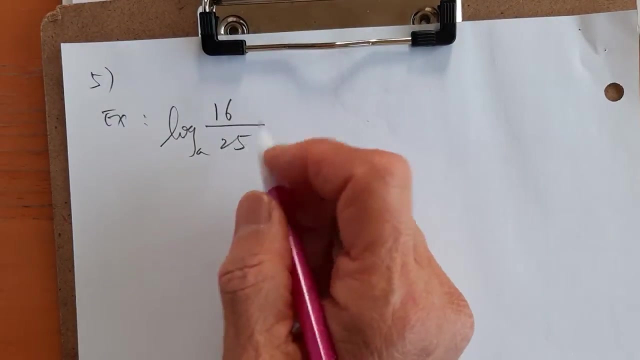 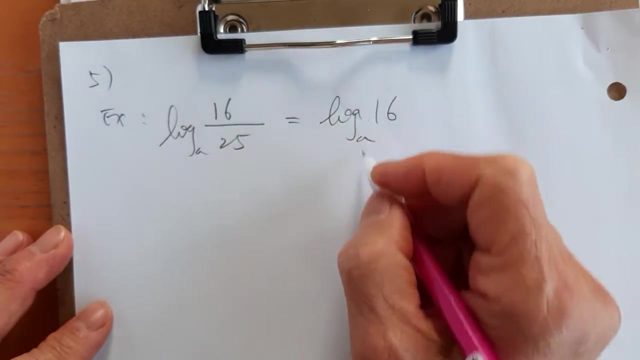 Divide This example. Example for homework, question 5.. Log 16 over 25.. 16 over 25.. You can use quotient rule, The quotient rule. Divide it, it becomes subtraction: Log 16 minus log Log 25.. 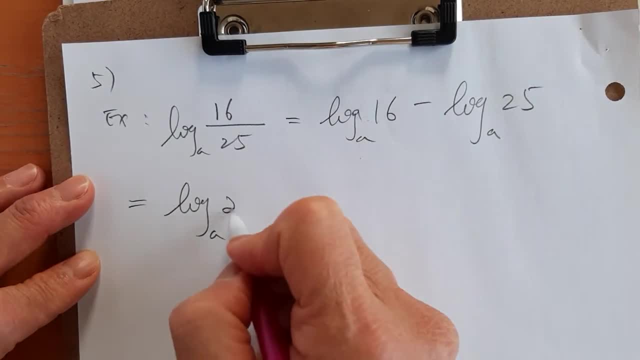 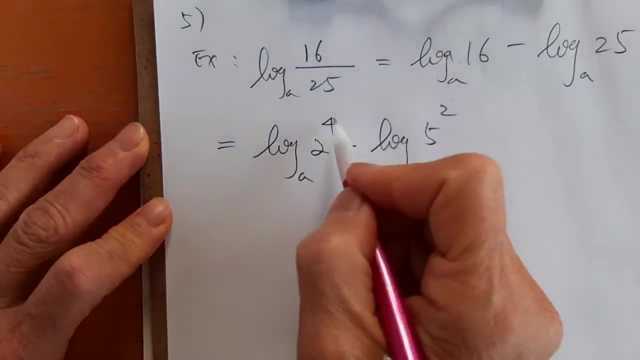 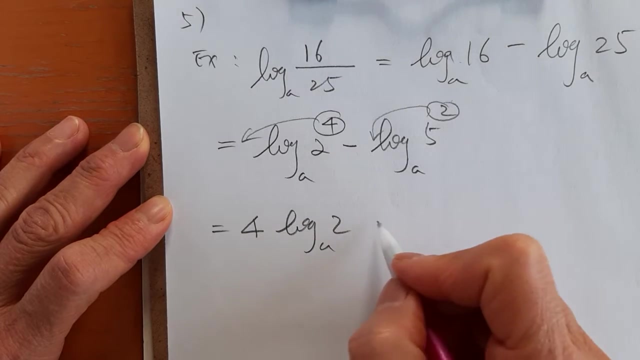 Then log 16 is 2 to the power 4.. 25 is 5 square. Then use power rule. This 4 go from, This 2 go from. So you got 4 times log 2 minus 2 times log 5.. 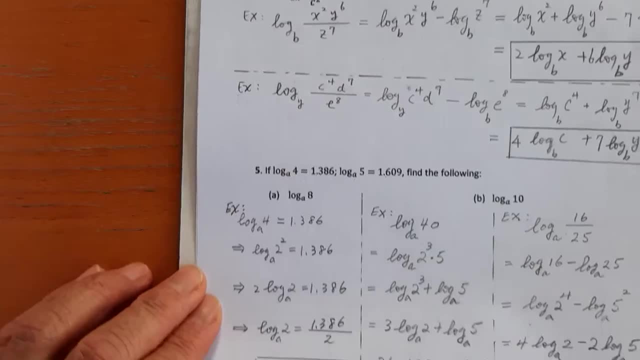 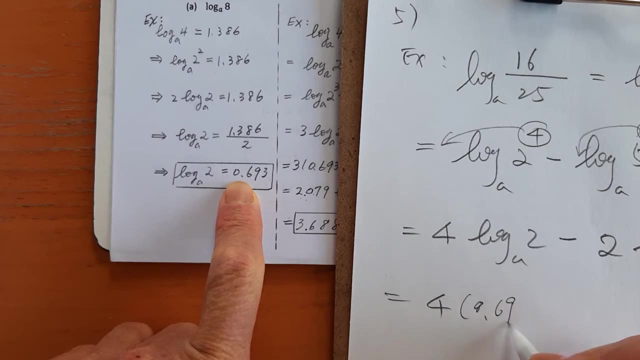 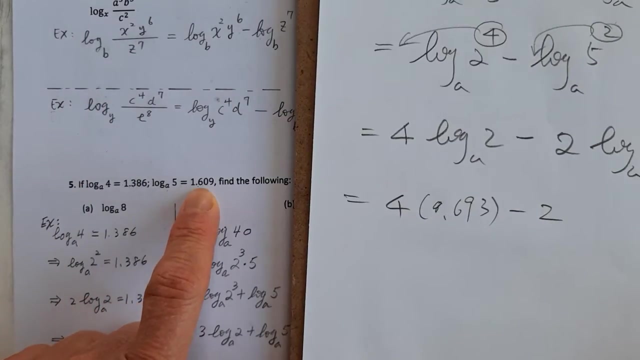 Now, what is the log 2?? That's from the. So the first example we got, log 2, is 0.693 minus 2, minus 2 times. what is log 5?? Log 5 is 1.609.. 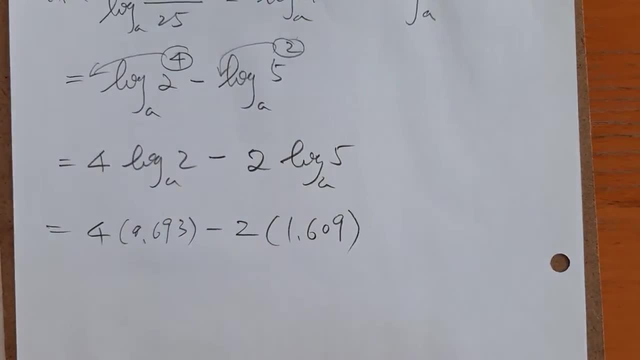 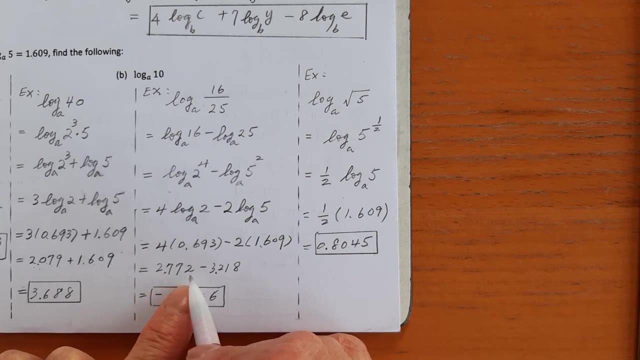 So log 5 is 1.609.. Then you figure out 4 times 0.693 and got is 2.772.. Minus 2 times 1.609.. Minus 2 times 1.609 is 3.218, and you will get negative 1,, negative 0.446.. 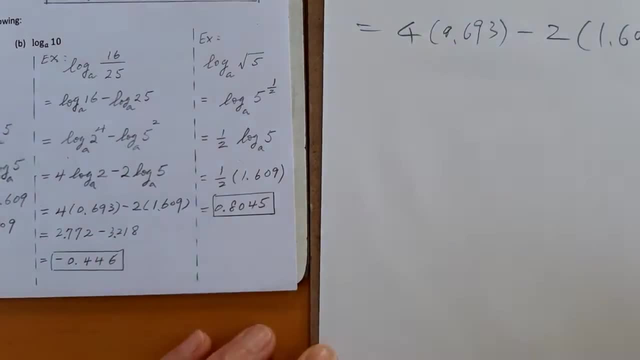 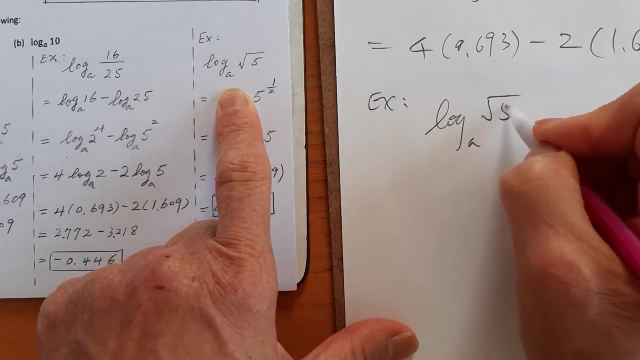 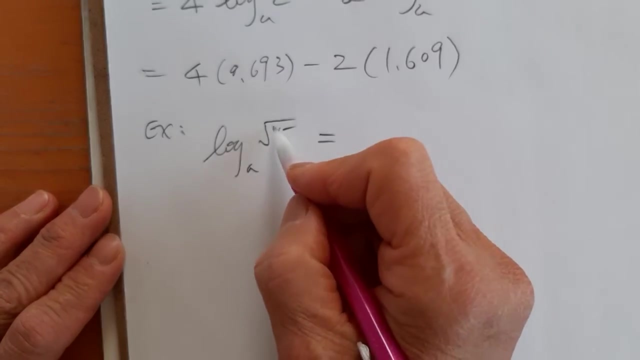 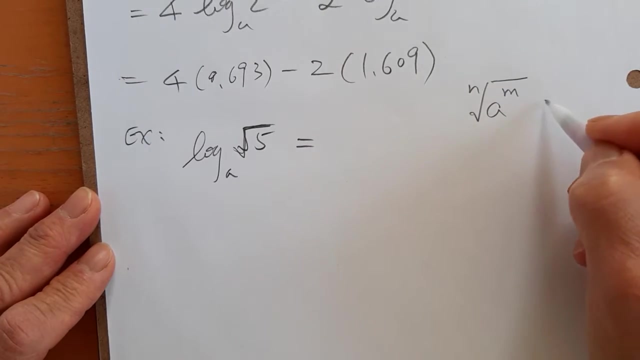 And next example. next example is this: one log: a square root of 5, square root of 5.. We can change this to radical form, to exponential form. Now use the formula a to the power m? nth root is equal. a to the power m over n. 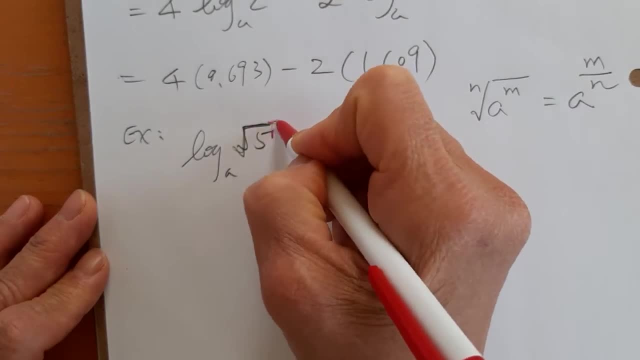 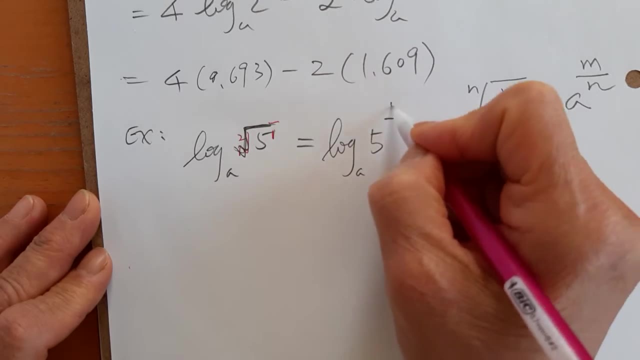 And this 5 means 5 to the power 1, and square root here means 2.. So you can change to 5 to the power 1 over 2.. m is 1, n is 2, m over 1, 1 over 2.. 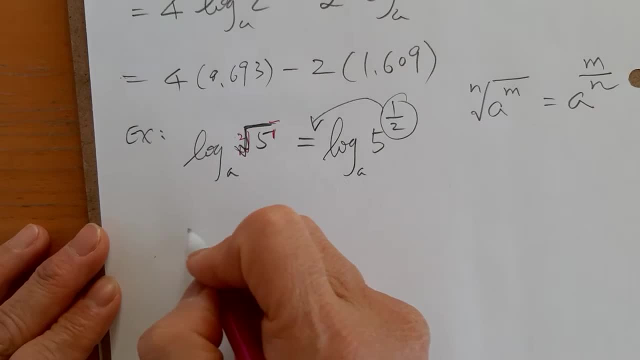 And then you go this use power rule This go from is 1 over 2, log 5, and you got 1 over 2 times and the log of 5 given is 1.609, 1.609.. 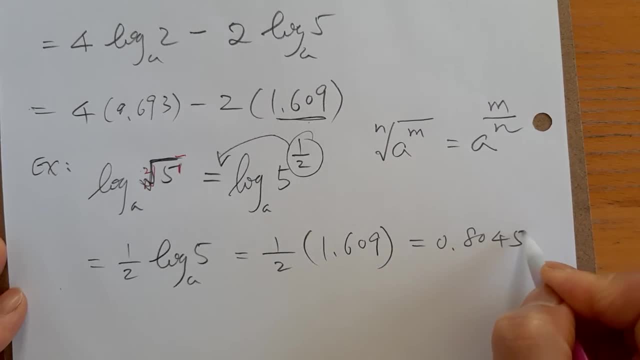 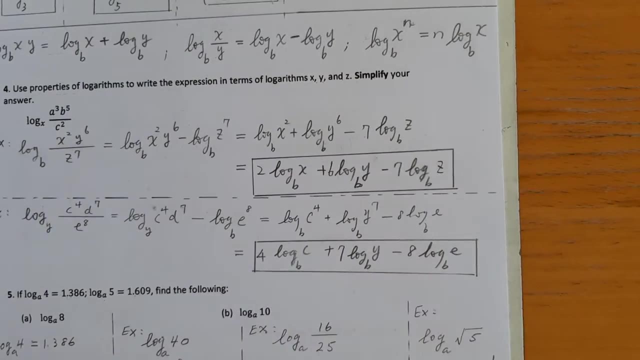 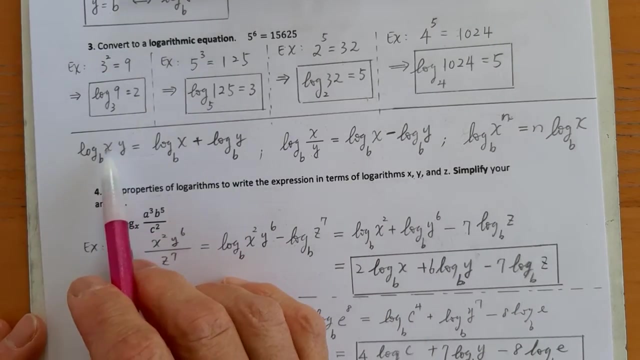 And you divide it as 0.8045, divided, just divided by 2.. So those are Prada rule we apply how to apply the Prada rule. We have a multiplication here: addition, Quotient divide, a quotient rule. you do subtraction. 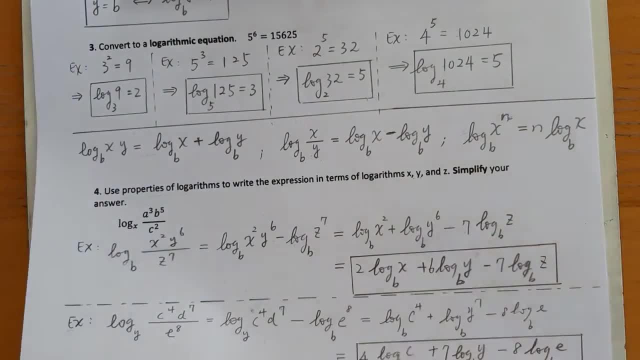 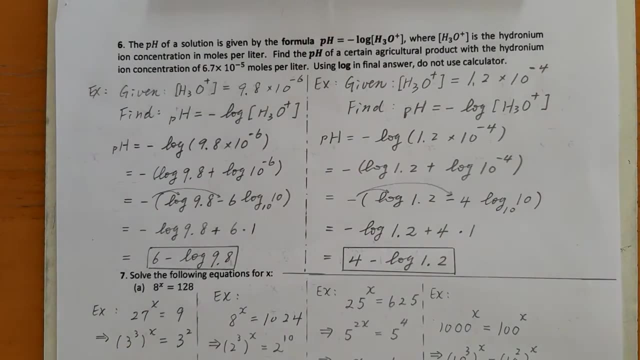 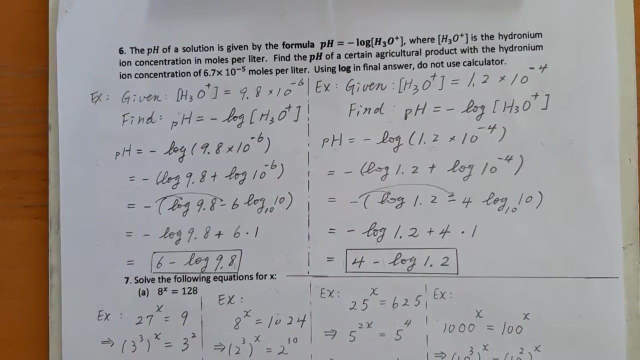 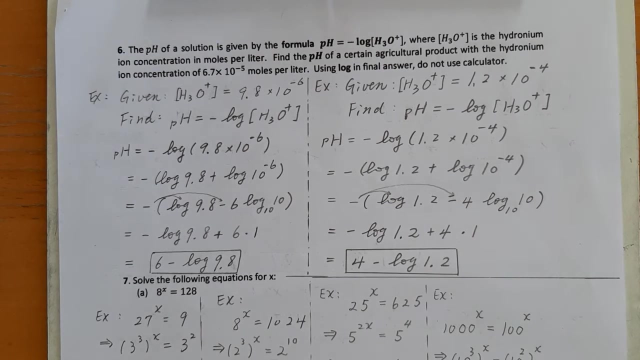 Then power rule. this exponent go from How. those is applications of the three rules. Then next is question 6.. Question 6, this is a word problem. A word problem Here, say the pH. chemical chemistry, The pH of a solution is given by the formula. 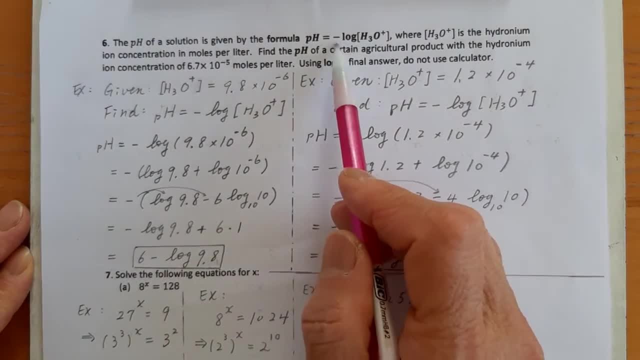 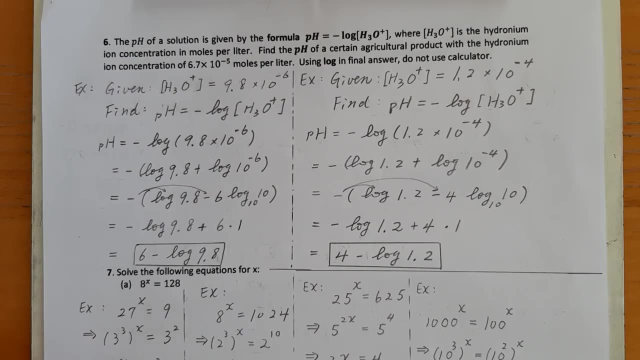 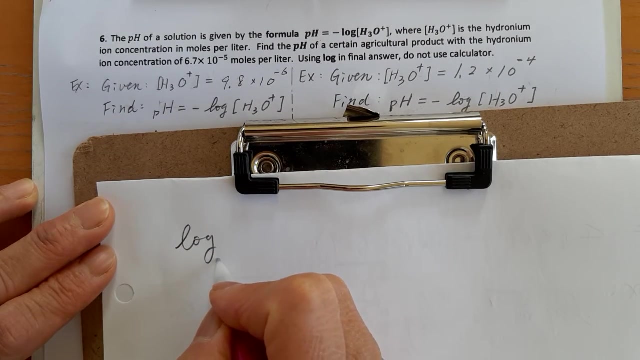 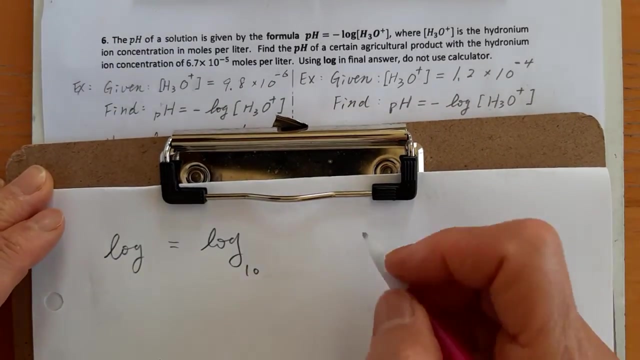 pH is equals negative log. And this log means: come on, I'm going to another. This log notation, If do not write down the base, Automatically means base is a 10. Base is a 10. Another, this one: 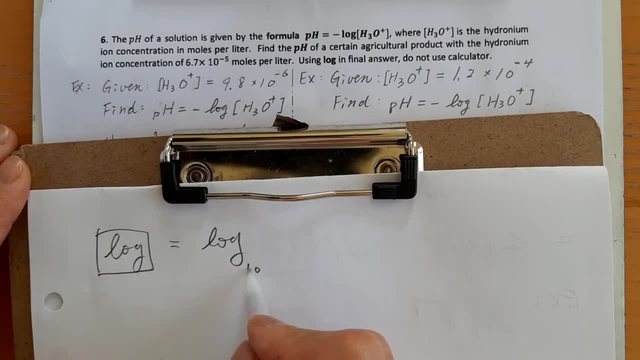 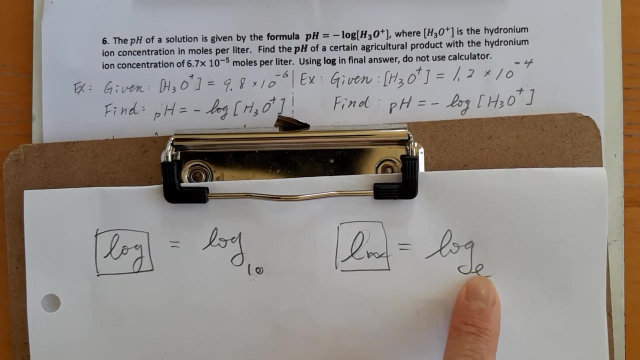 In calculator you have this key. It means base is a 10. Another one is ln. ln means natural E. E is a natural number, natural number. So ln n is natural. E is a natural number, natural number. 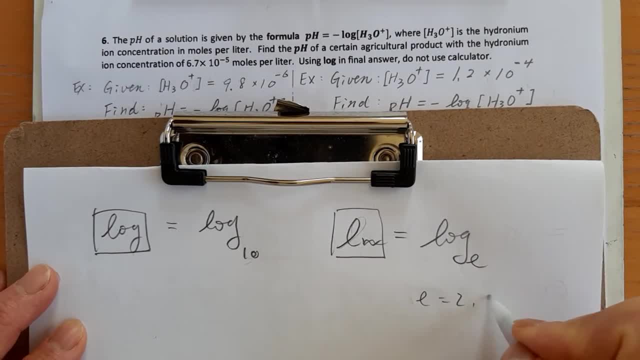 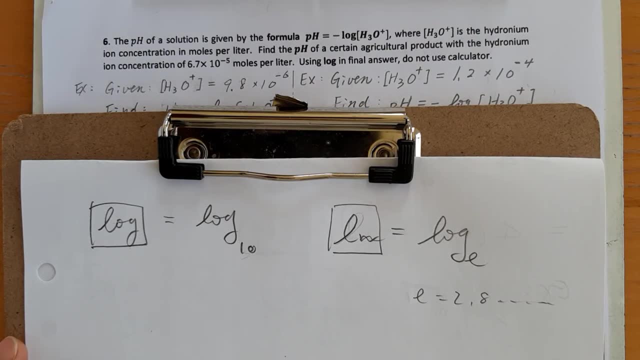 Means base is E. E is about 2.8. something Is a irrational number Is: keep going on, One, non-terminating, Non-stopping. The decimal digits keep going on. So this is two kind of notation. 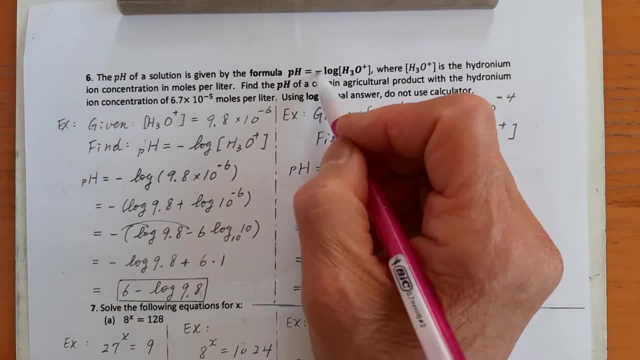 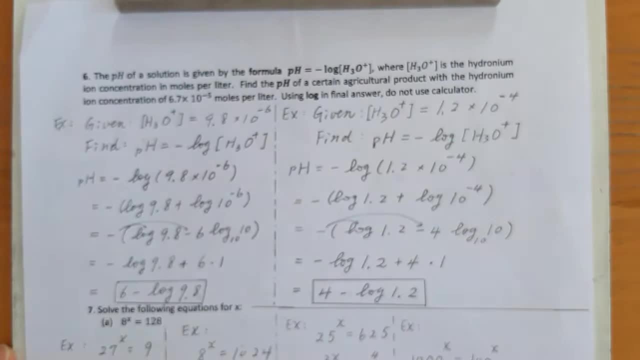 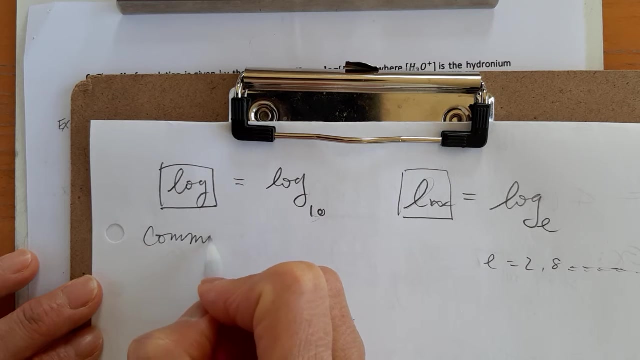 And this question here: say pH equals negative log. This do not put down. the base Means: base is a 10. Base is 10. This we call common log reason. Base is 10. This we call common log reason And the base is E. 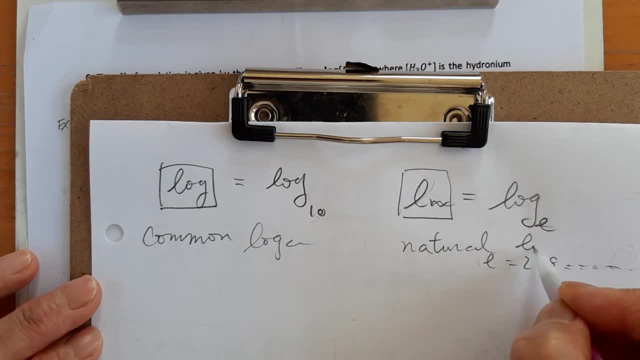 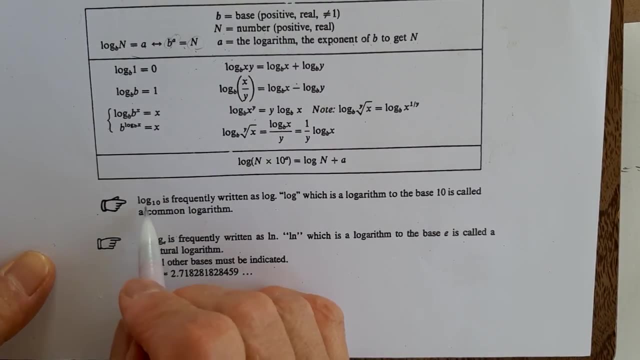 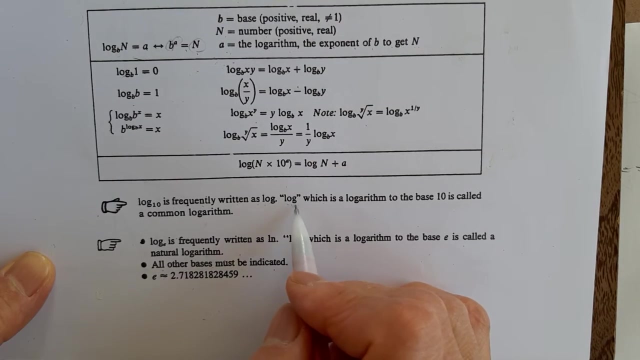 We call natural Natural log reason. Natural log reason- You can see this in your notes. Log base is 10- is frequently written as just log Log, Which there is no put down. the 10. Means base is 10. Which is a log reason. 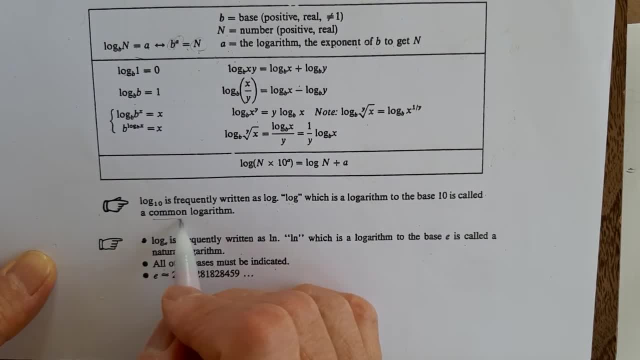 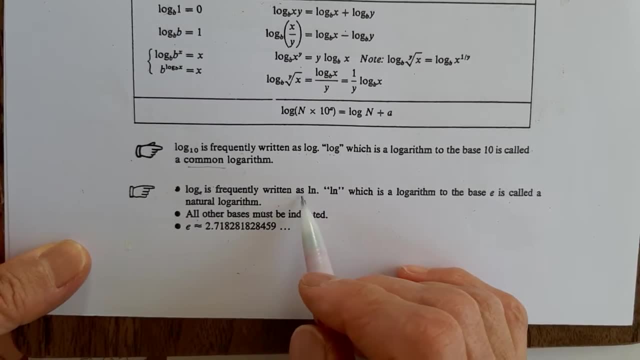 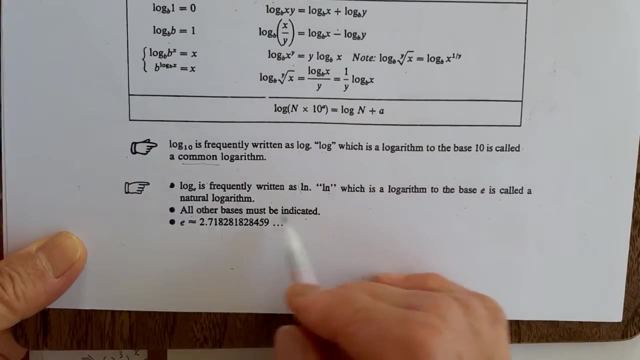 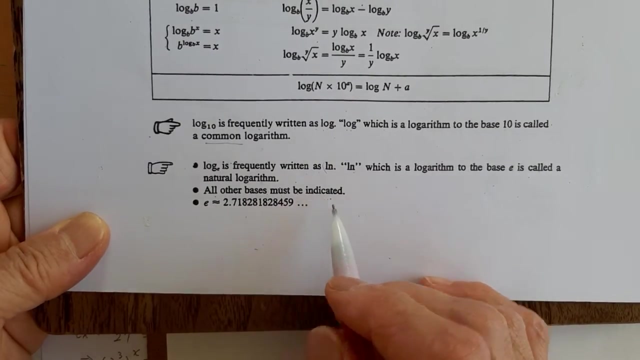 To the Base 10 is called common log reason. This is called common log reason And log, if base is E, is frequently written as Ln, Ln, which is a log reason. to the base E is called natural log reason And all other bases must be indicated. 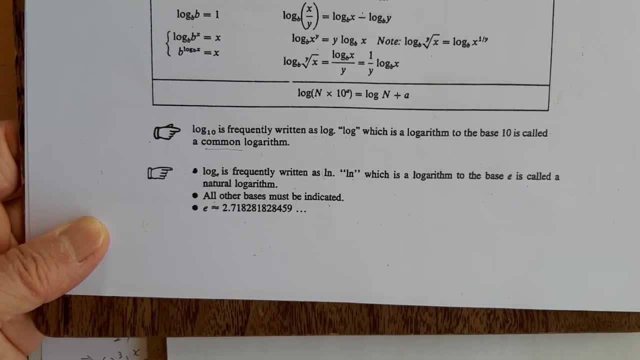 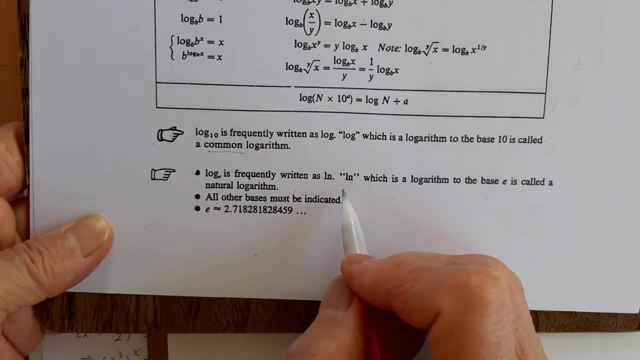 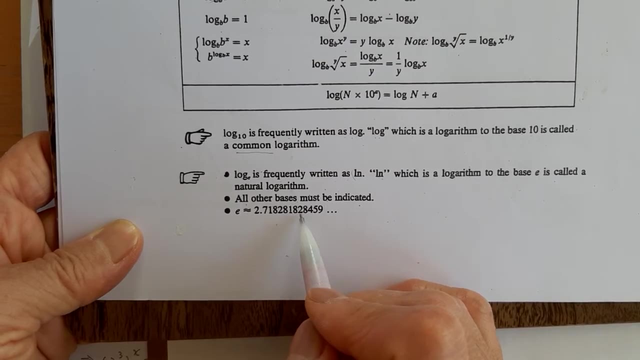 All other bases must be indicated. Only the base is 10.. You can just put log. If base is E, you write down Ln. What is E, E is 2.71828.. Keep going on Non-stop, Non-terminating. 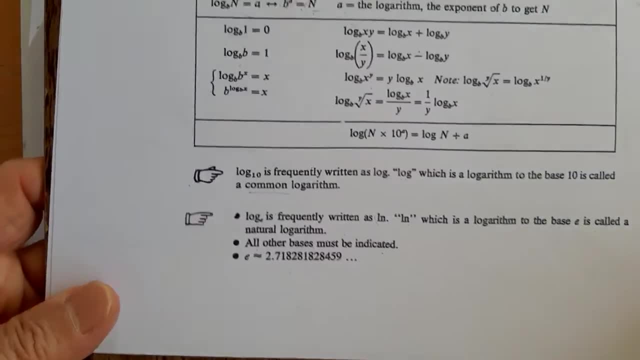 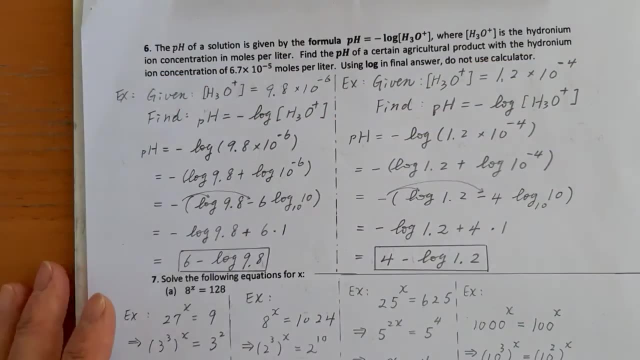 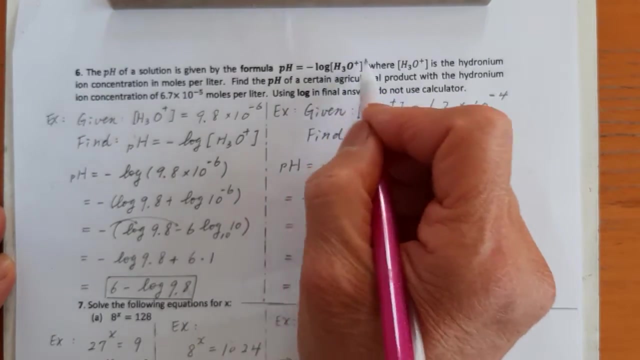 Non-repeating. It is an irrational number. It is a real number But irrational. So this question, So this question Here. do not write down the base Log means 10.. The formula pH value equals negative common log. reason of this: H3O plus. 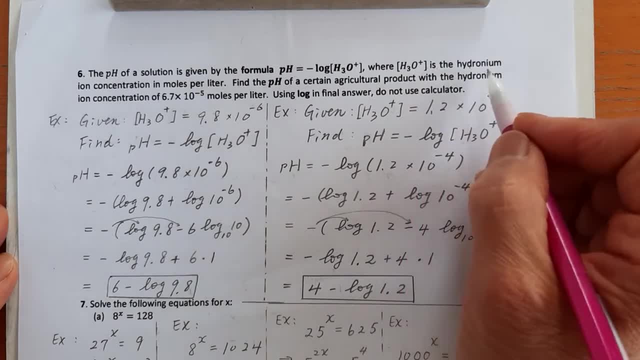 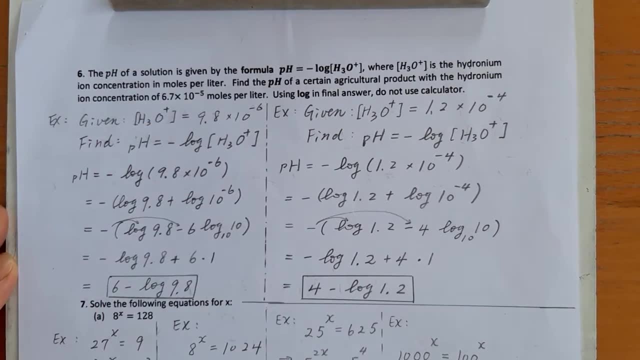 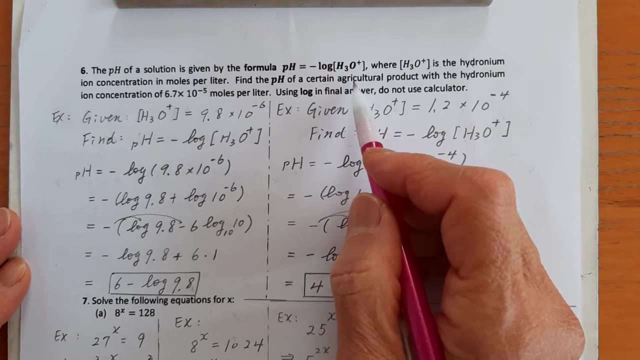 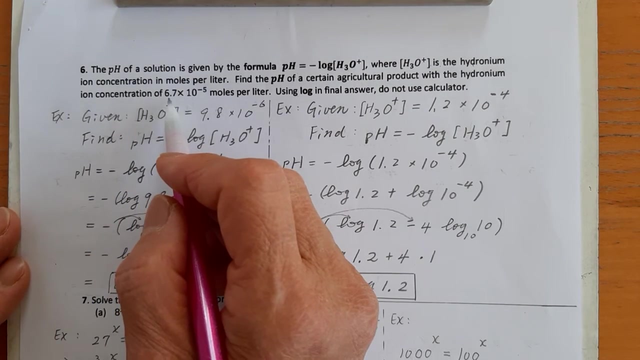 This is H3, plus is the hydronium iron concentration And in moles per liter And find the pH of a certain agriculture. And find the pH of a certain agricultural product With the hydronium iron concentration of 6.7 times 10 to the power negative 5 moles per liter. 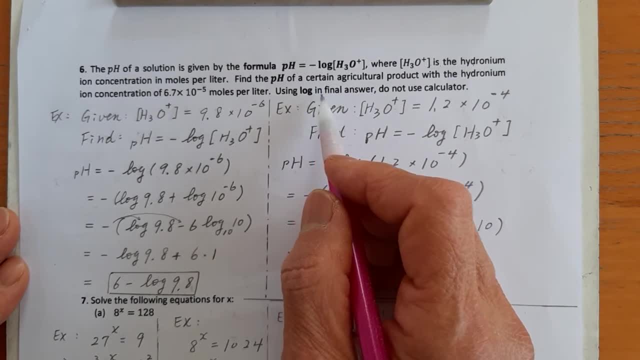 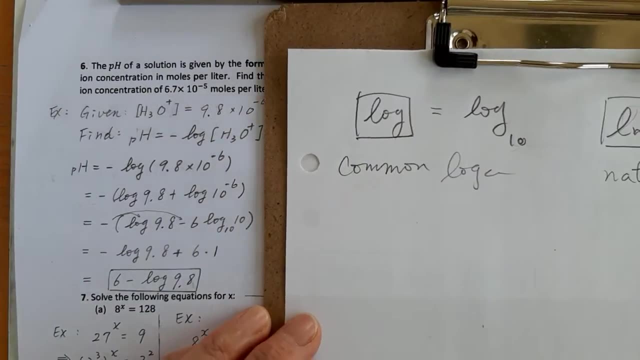 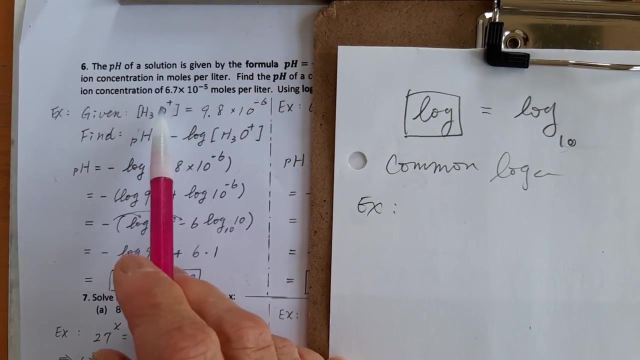 And using log, Common log. reason in final answer: Do not use calculator to figure out. Do not use calculator to figure out. So I give you one example. So I give you one example. I give you one example. If H3O plus a, hy некоторые. if H3O plus a. 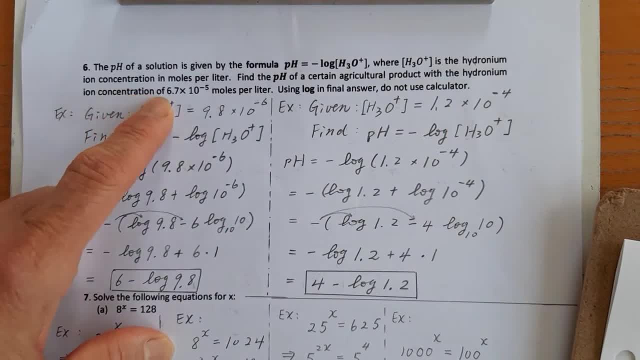 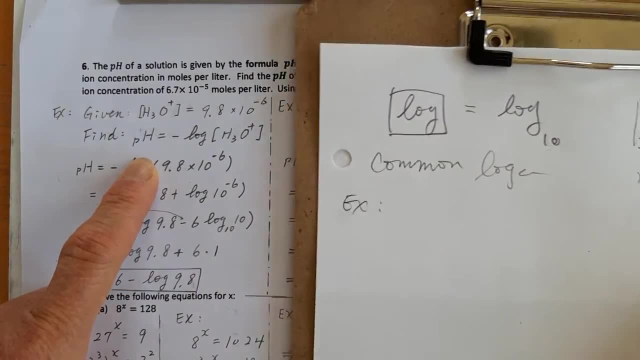 hydronium Hydronium iron concentration. Hydronium iron concentration is 9.8 times 10 to power negative. 6. Find out pH value. So pH value equals negative log. So pH value equals negative log. 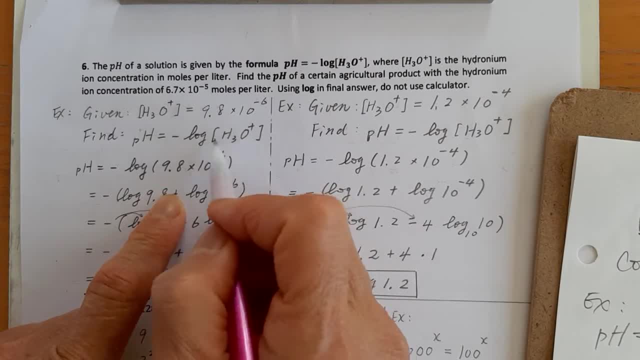 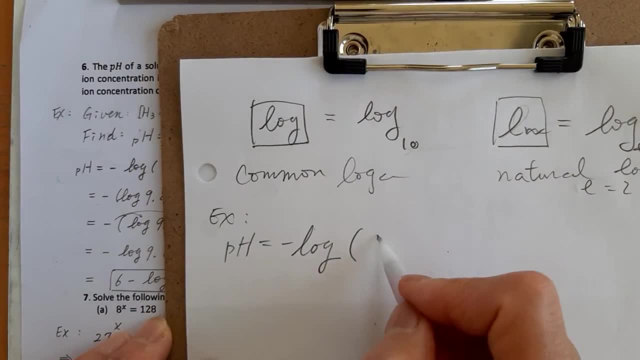 And this part, This iron concentration, is subtd by 9.8 times 10 to the power negative 5.. times 10 to the power negative 6 substitute in. so it's a 9.8 times 10 to the power negative 6. 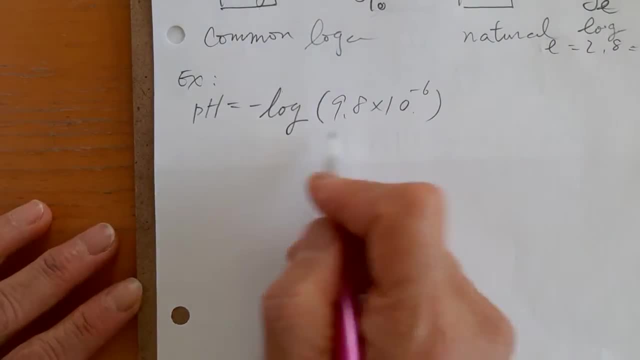 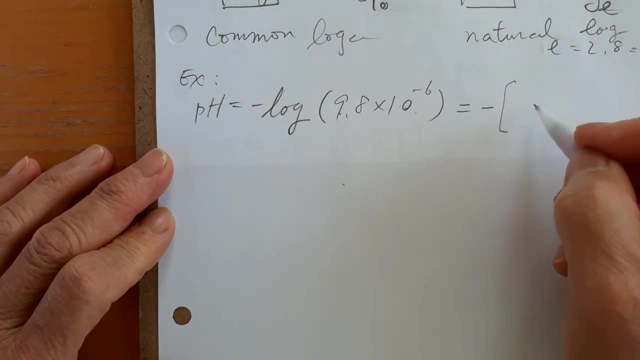 is the iron concentration and figure out this now. this one is equals negative product rule. put down the bracket or parentheses. log common logarithm. do not put down 10, 9.8. add product rule. so add log 10 to the power. negative 6 x times y, the two times together. 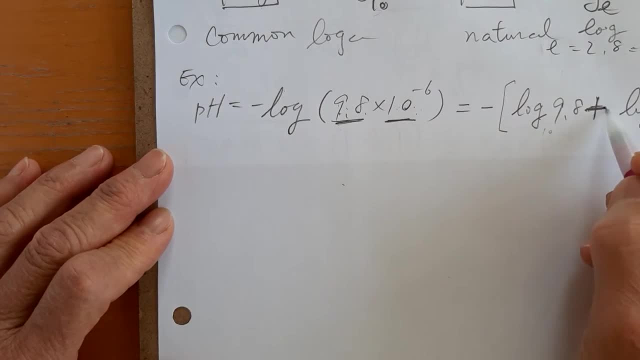 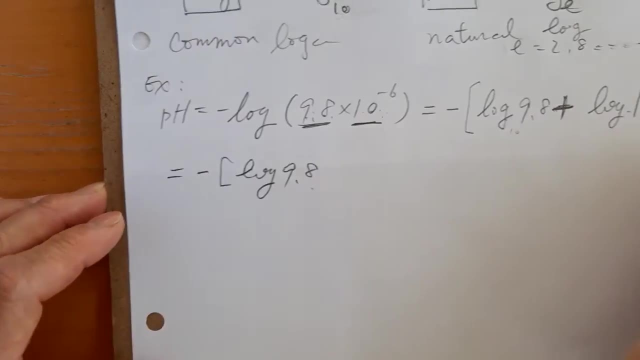 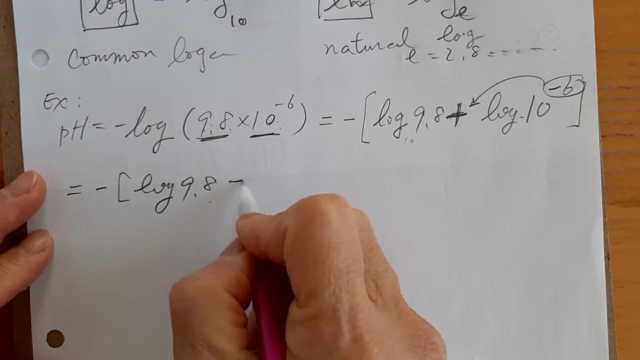 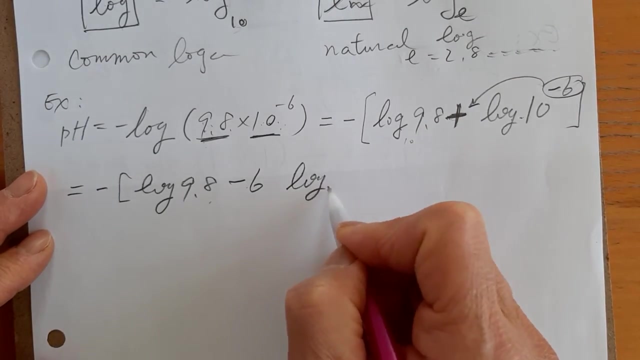 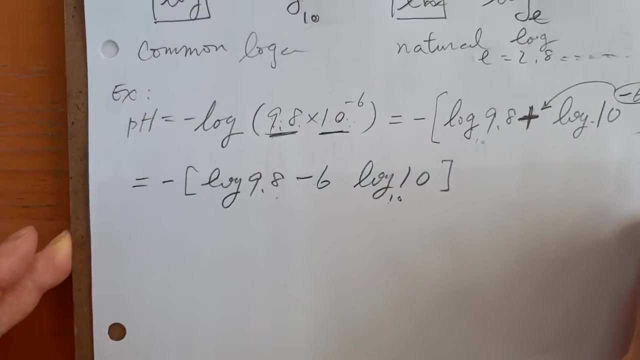 equal the two separate. take logarithms and add together. so equals negative log 9.8 and this negative 6 go power rule: go from got minus 6 negative 6 times plus is a negative 6 log 10, 10.. the base is 10.. so then use distributed property. 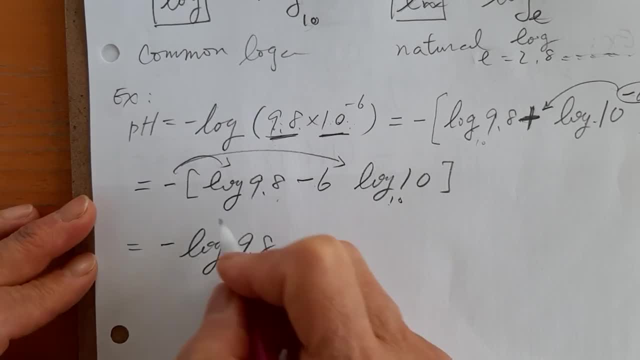 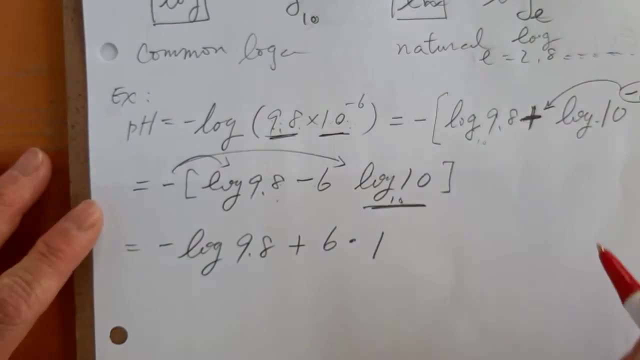 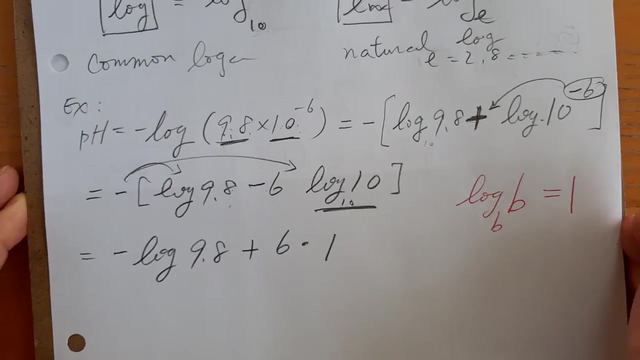 so you got net log 9.8 negative times. net become plus 6 times this one equal one. so there's another formula: log: if base is b, b will be 1 because because b to the power, 1 equal b. so 10 log 10: 10. 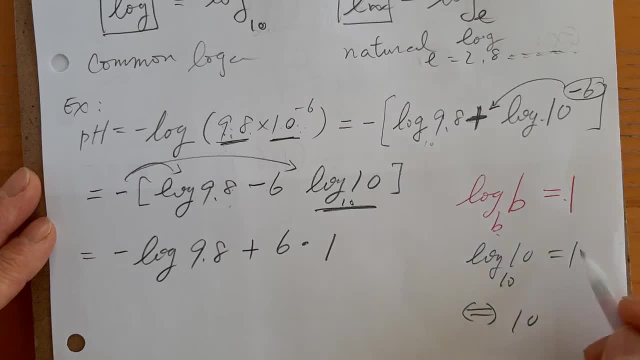 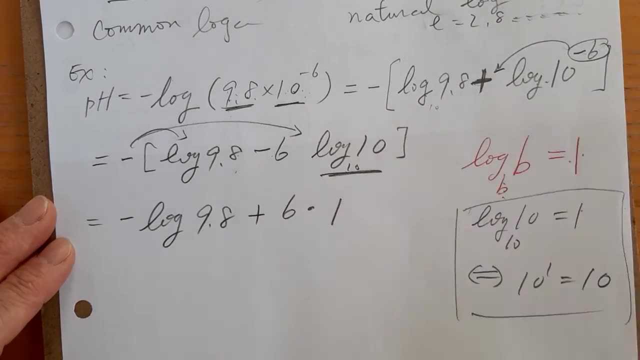 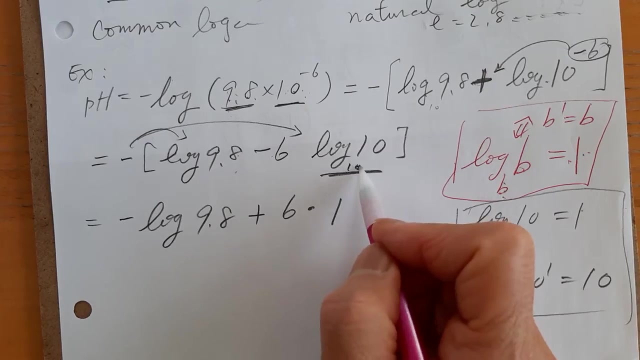 equal 1 because because 10- 10 to the power 1 equal 10 equivalent. this also b to the power 1 equivalent. this is the equivalent to b to the power 1, equal b. b to the power 1, equal b. so log base is b b is equal 1. so log base is 10: 10 equal 1. 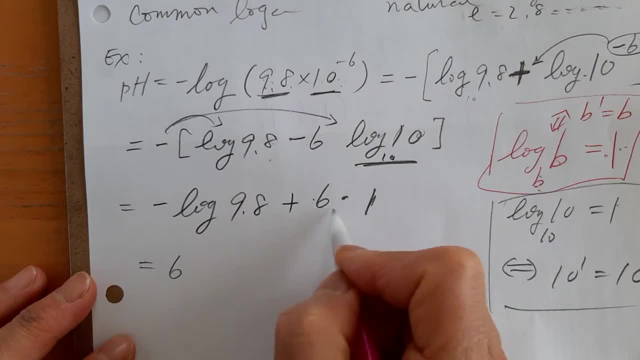 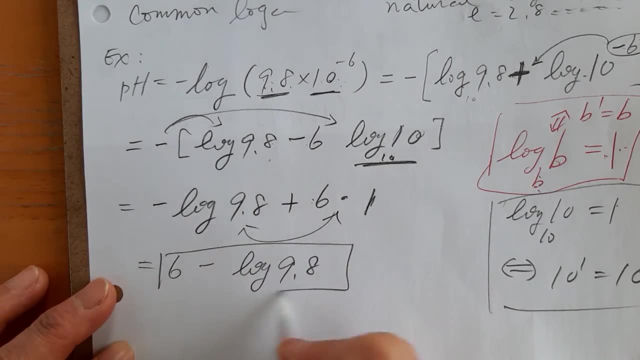 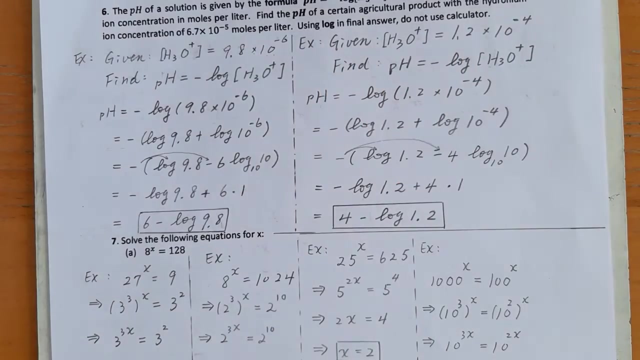 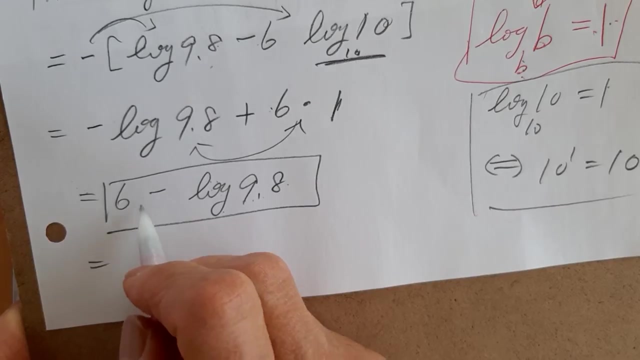 so then this 6 times 1 is a 6. you can exchange the order become 6 minus log 9.8. and that's the final answer. because here question say: use log. in final answer: do not use calculator. if, if you want decimal, you can use calculator, figure out log 9.8 and subtract from 6, you will. 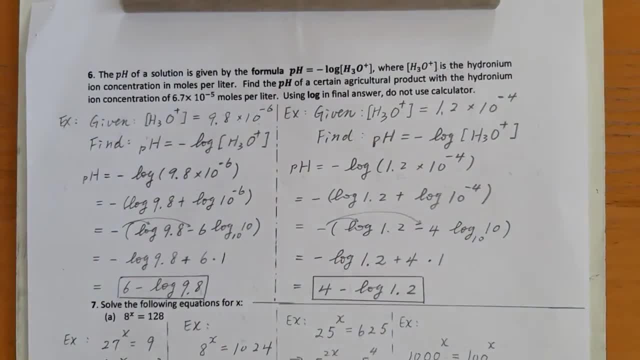 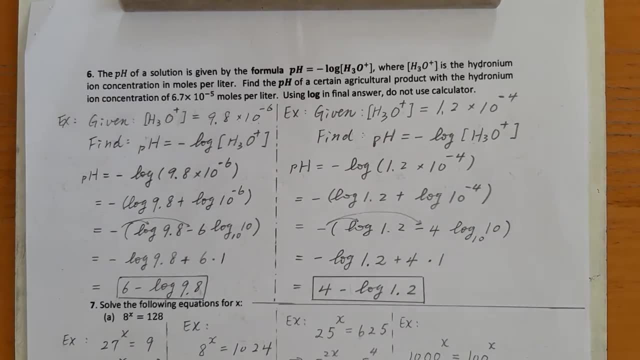 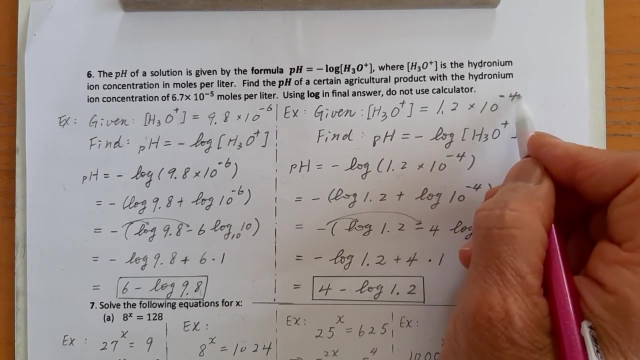 get a number but here one just leave, like that you don't need to use calculator to continue figure out. uh. next question: if uh given uh uh example, uh, question hole six. another second example: if, given the iron concentration is 1.2 times 10 to the power, negative 4. then you put this number into. 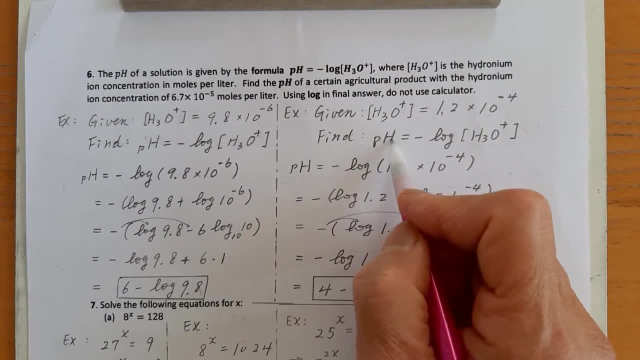 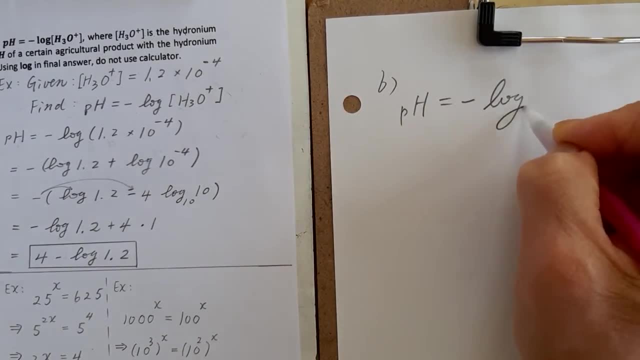 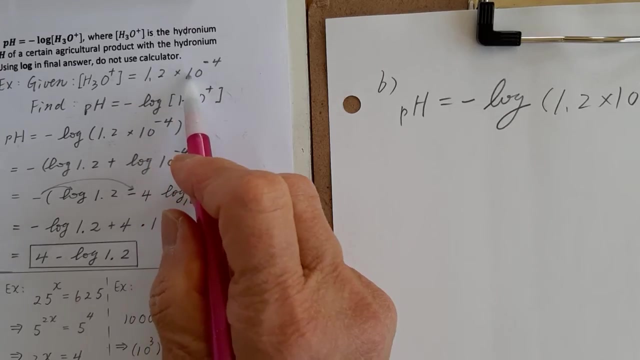 into log into here. so p find ph value. so your ph value is equals negative log and then, given the number is 1.2 times 10 to the power negative 4.. 1.2 times 10 to the power negative 4, put it in here and figure out ph value. so this one. 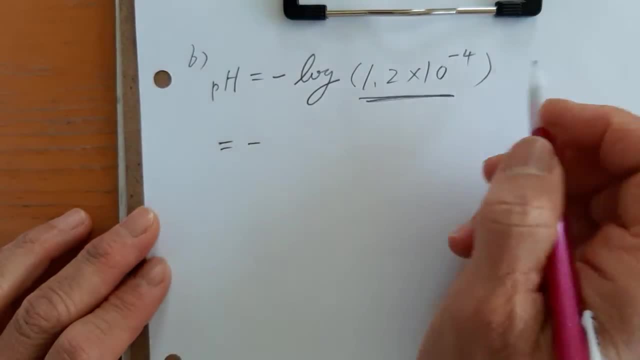 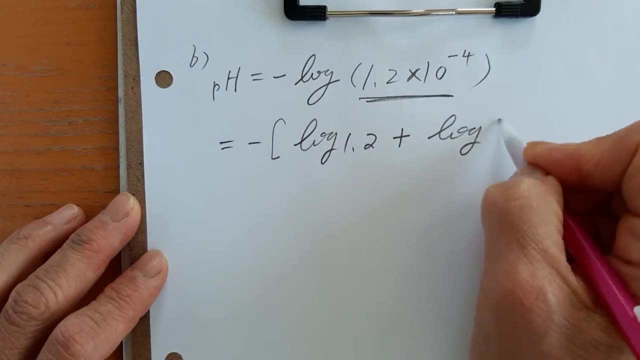 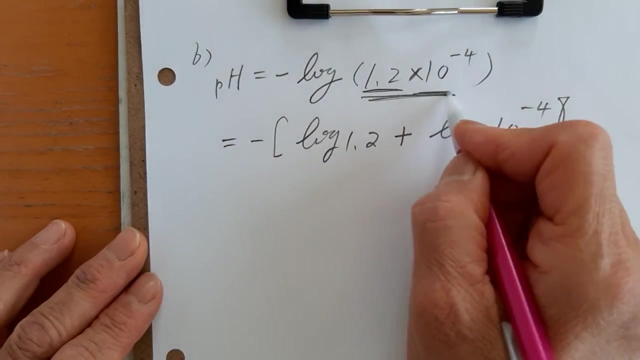 is equal to negative product rule. here's multiplication: become log 1.2. add log 10, negative 4, then you put this in here and you divide this by a 1.2 and then you add 2 to the 2 and then you: 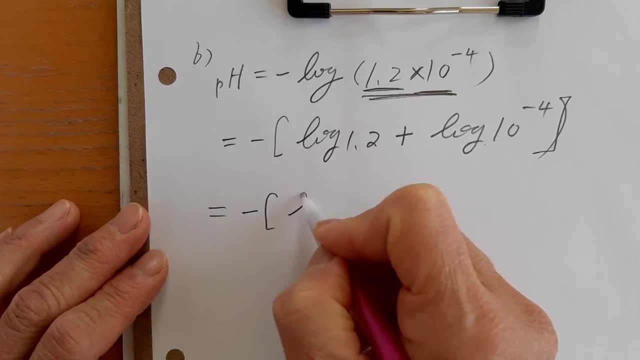 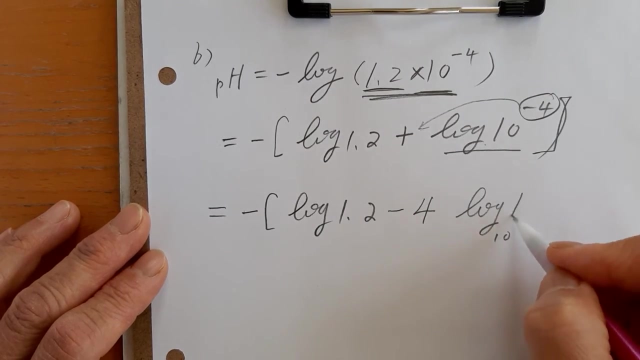 add, uh, add together, then, uh, negative log 1.2. then use power rule this negative 4 go from times positive, become minus 4.. and this means a log base is 10, 10 base is 10, do not write out, it's 10.. common logarithm. 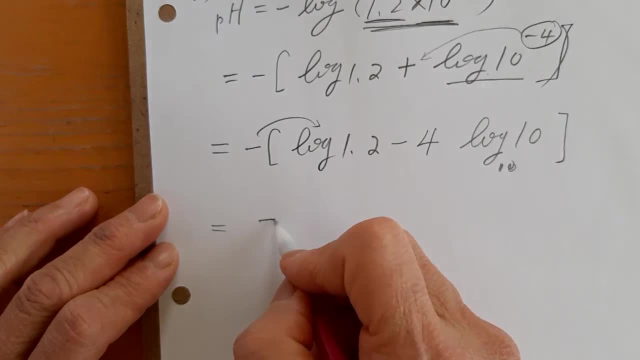 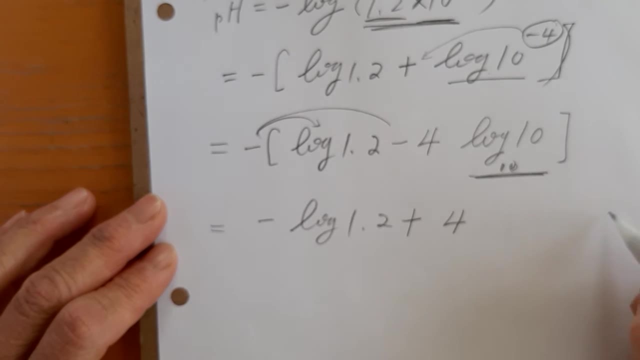 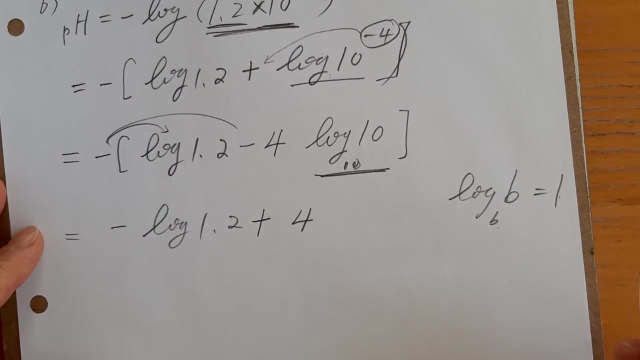 And then this becomes distributive n, negative log 1.2, negative times, n becomes plus 4.. What is log 10, 10?? Because log b, b equals 1.. b to the power, 1 equals b. So then log 10, 10 equals 1..